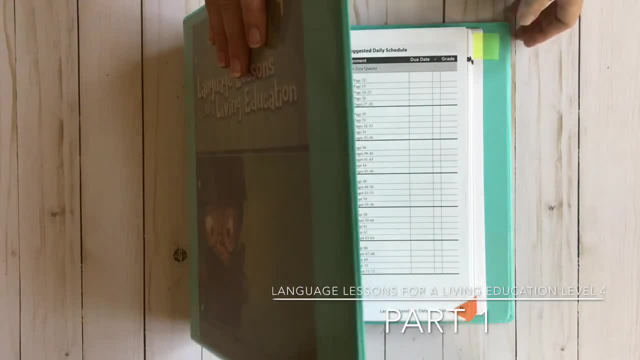 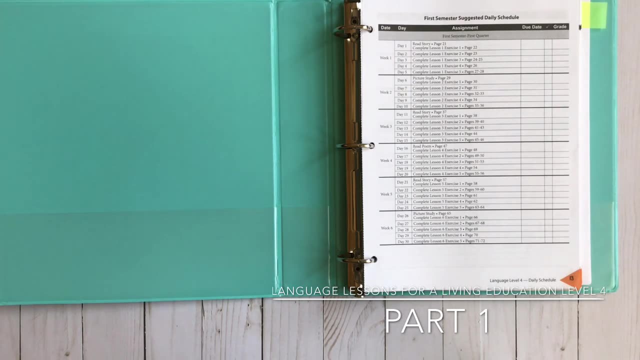 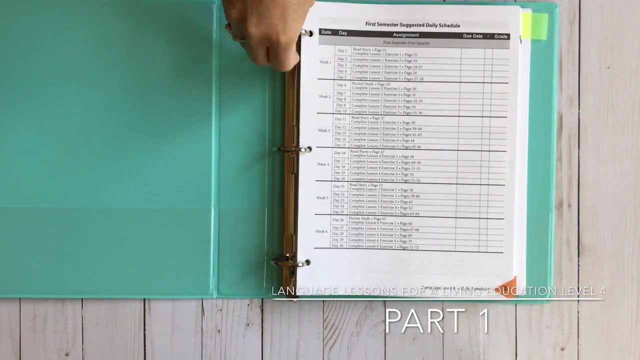 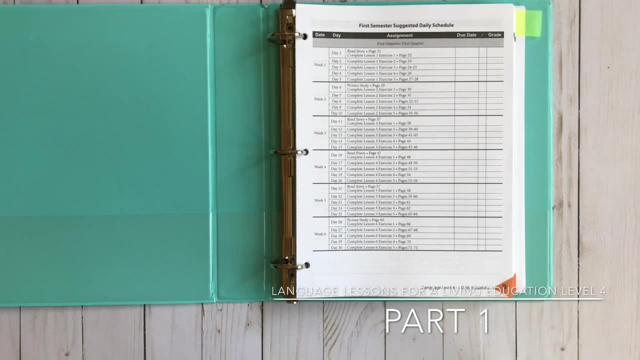 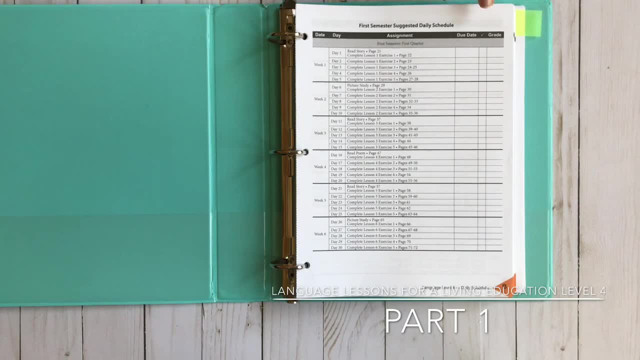 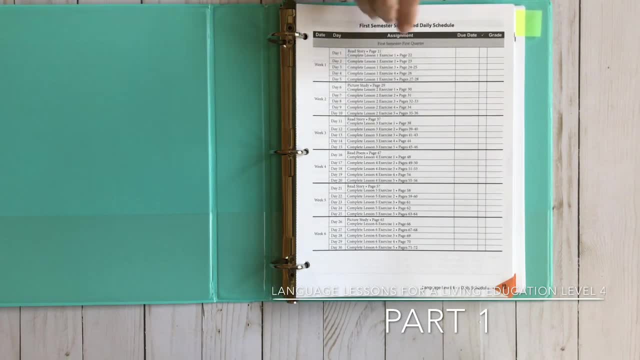 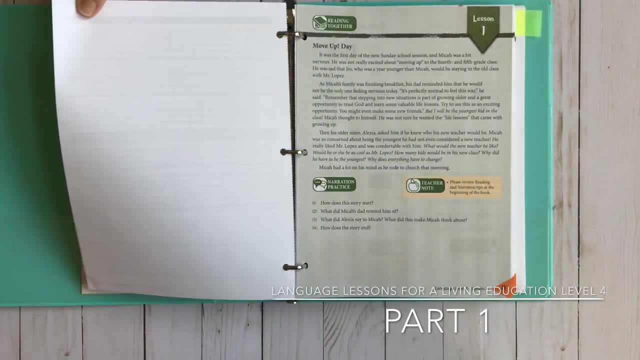 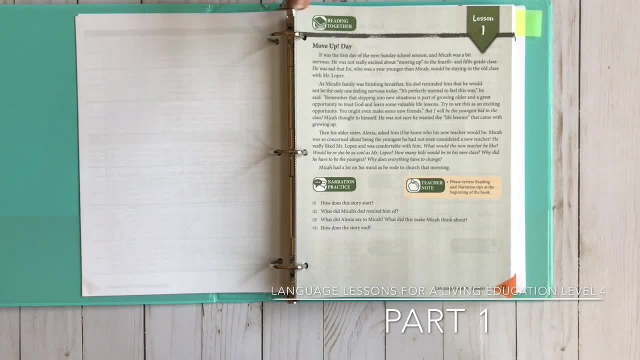 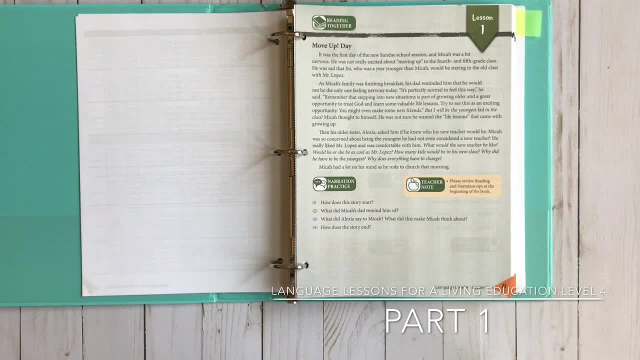 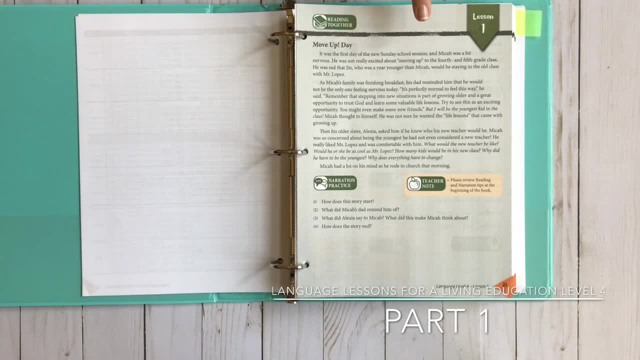 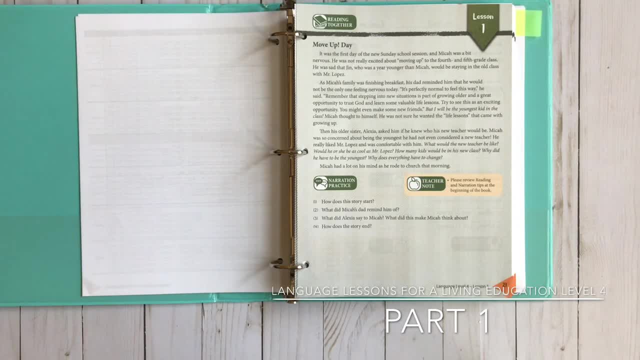 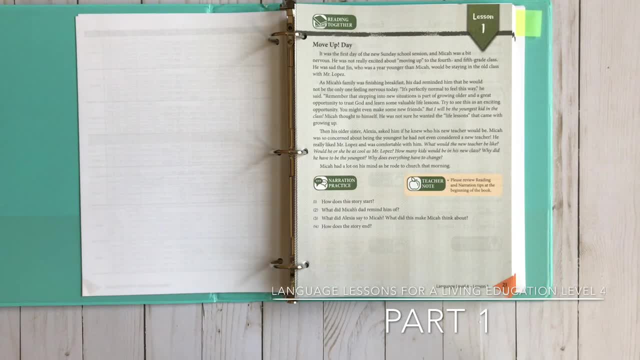 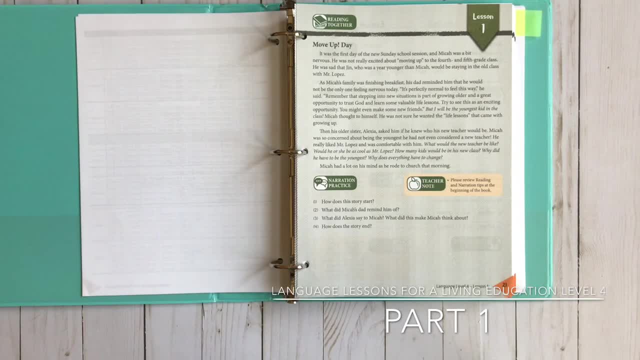 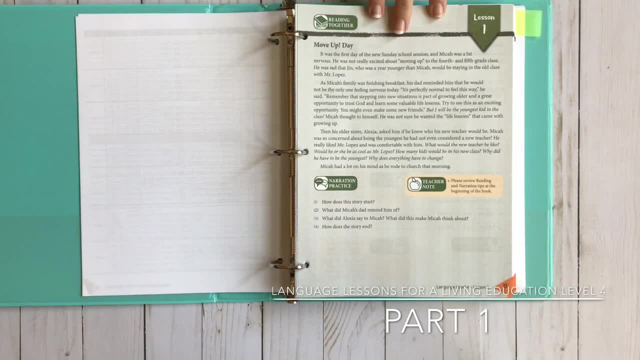 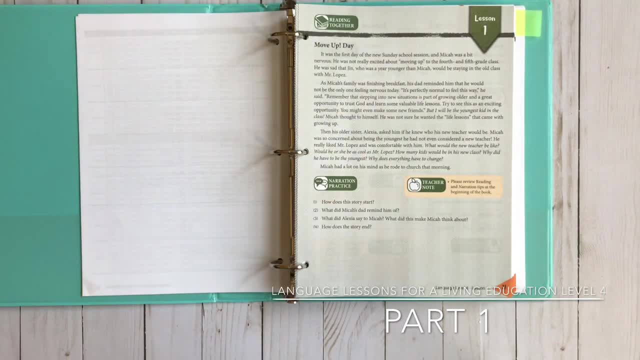 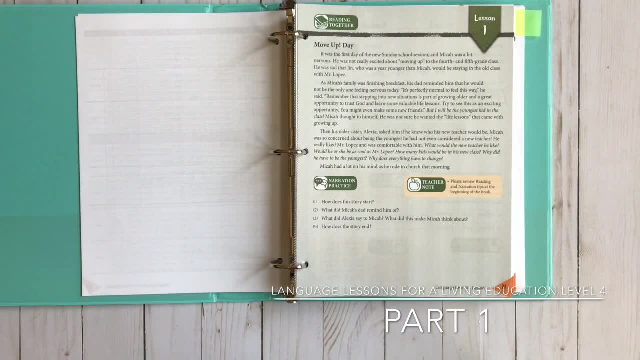 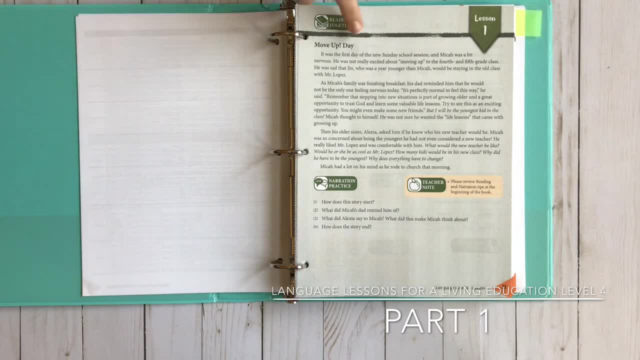 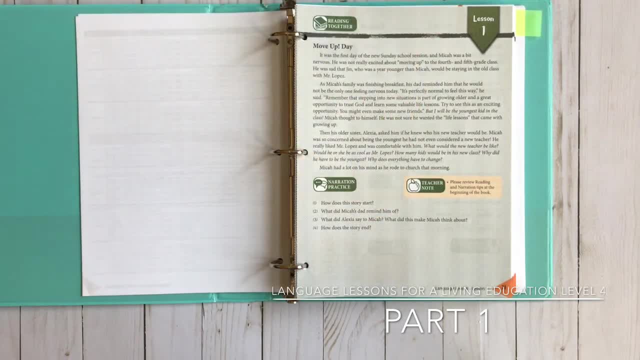 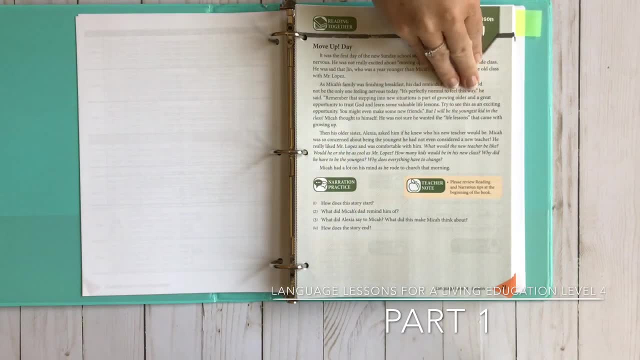 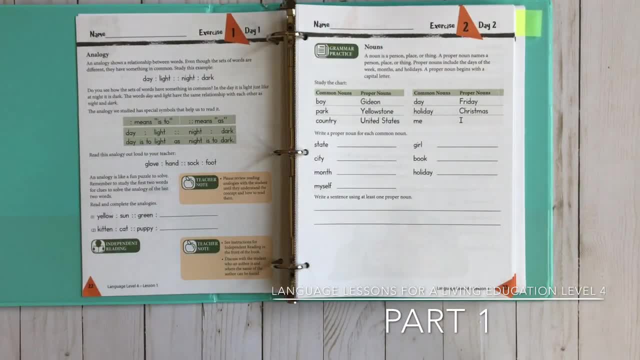 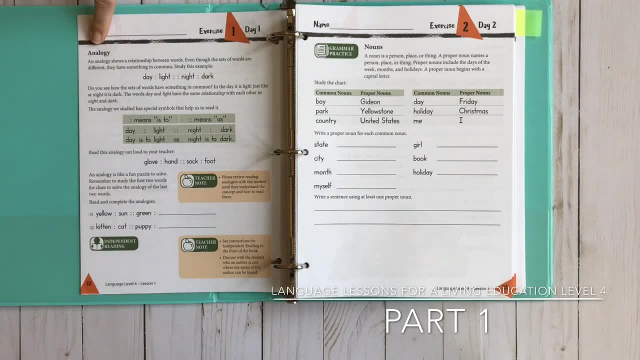 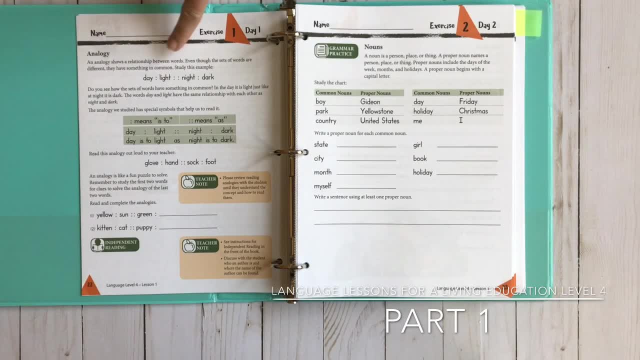 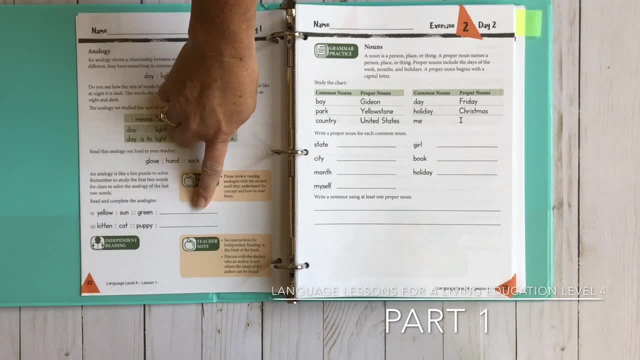 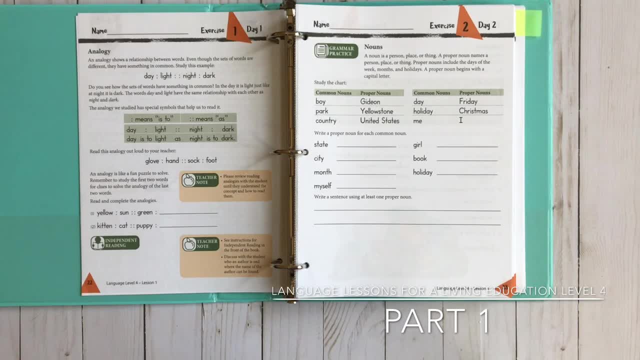 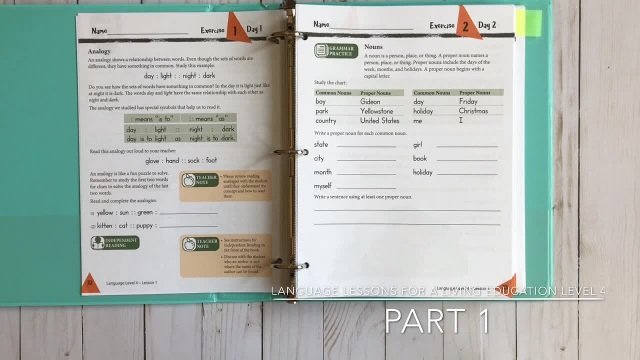 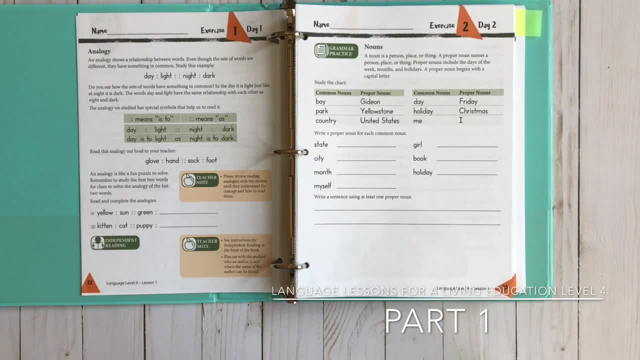 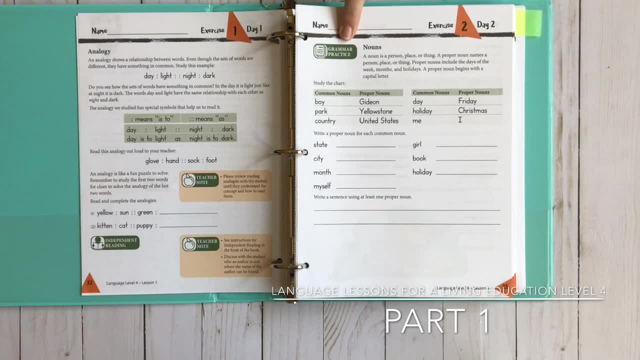 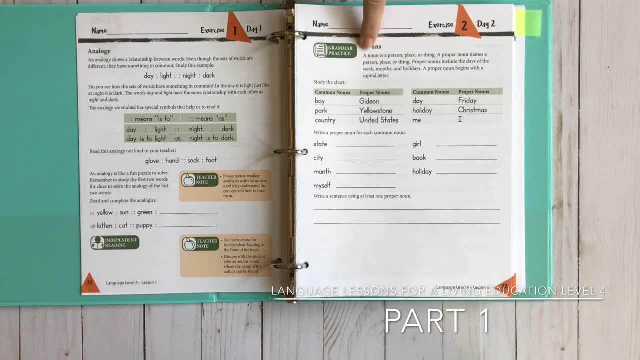 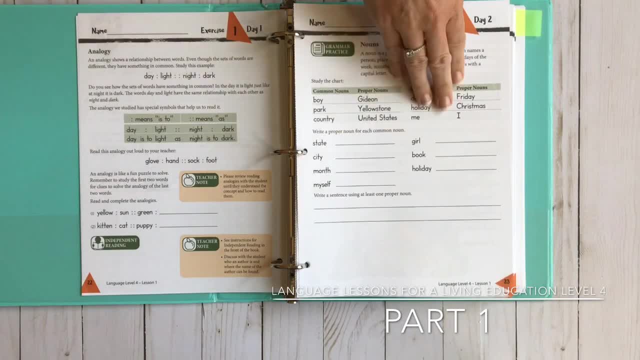 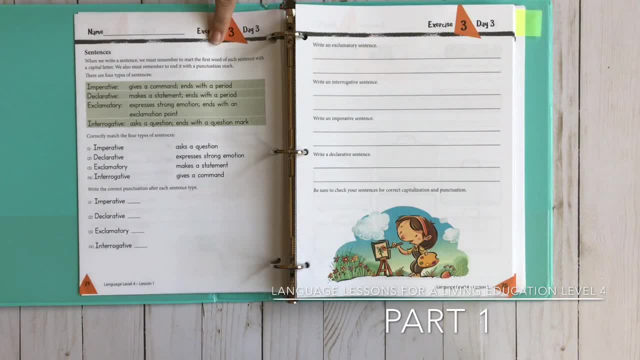 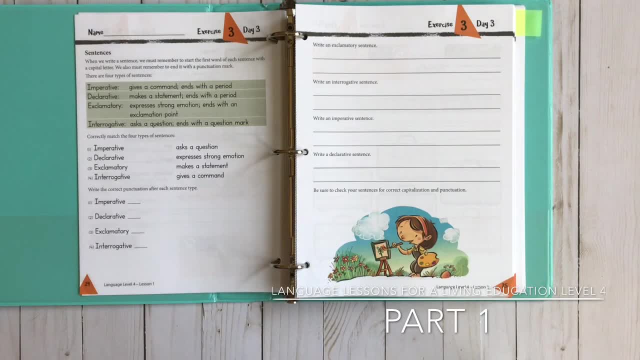 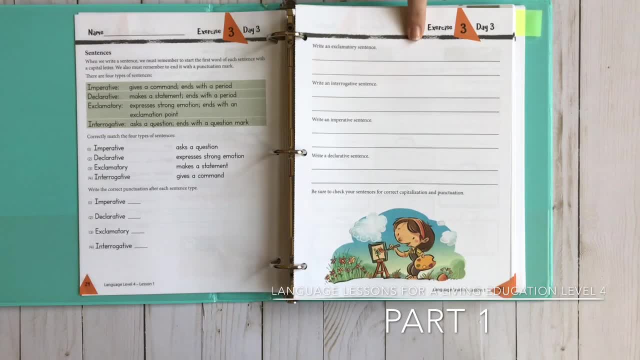 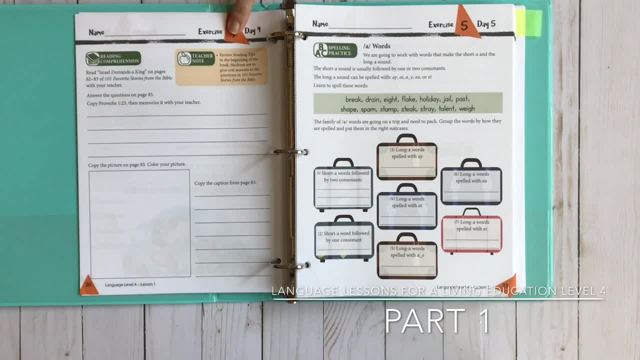 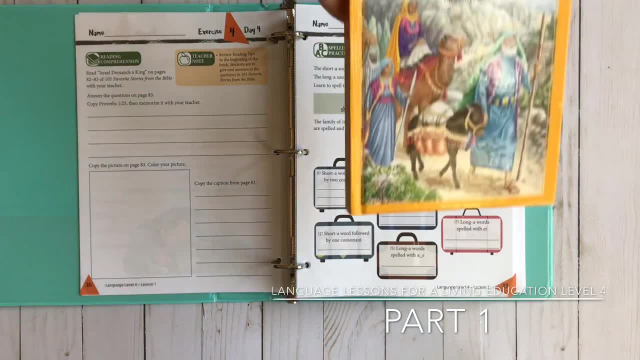 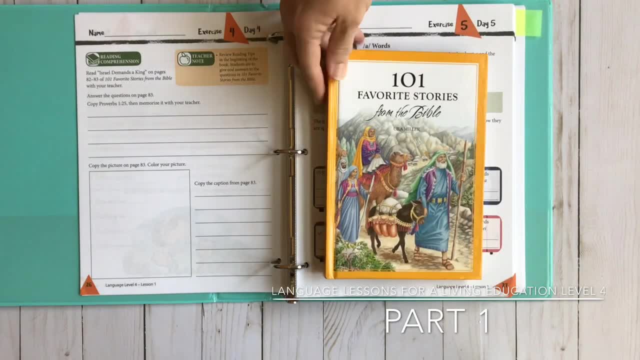 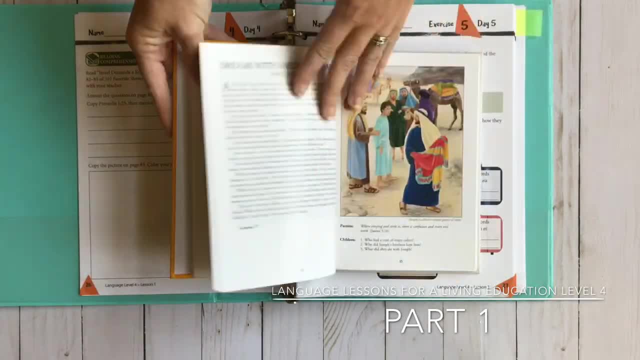 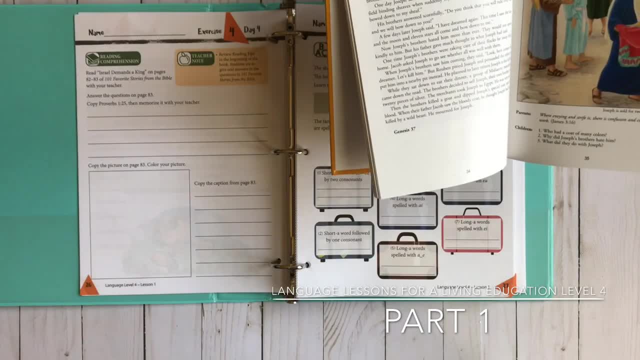 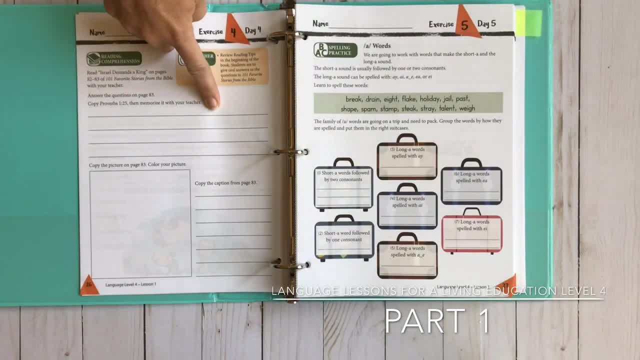 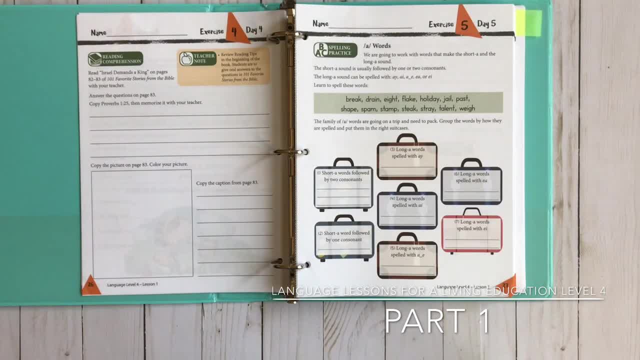 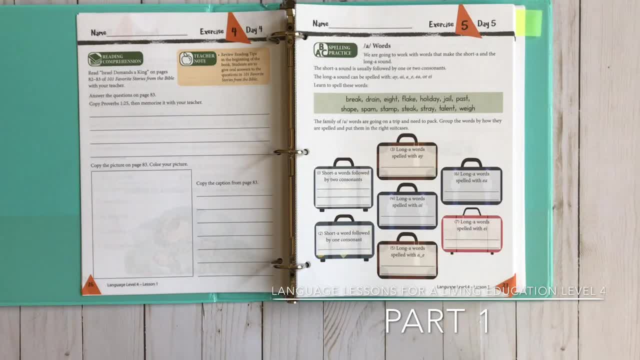 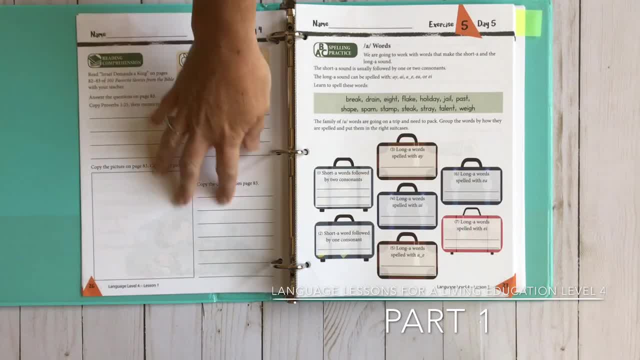 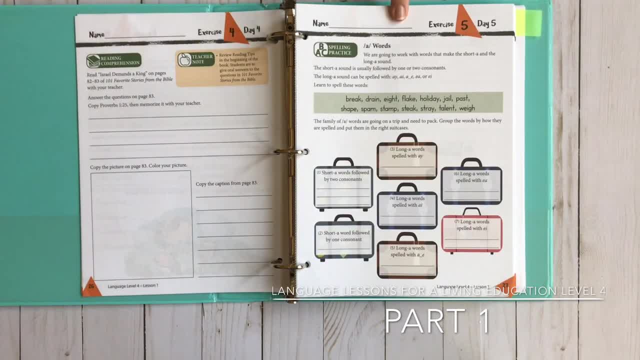 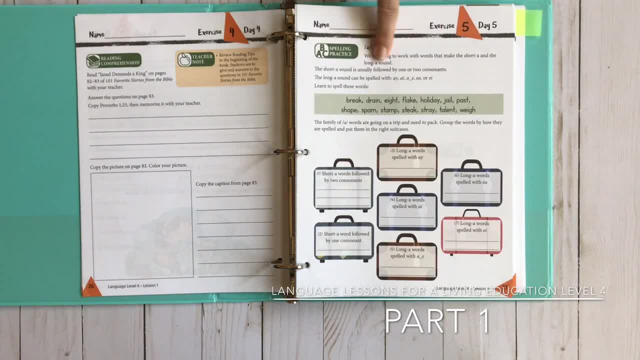 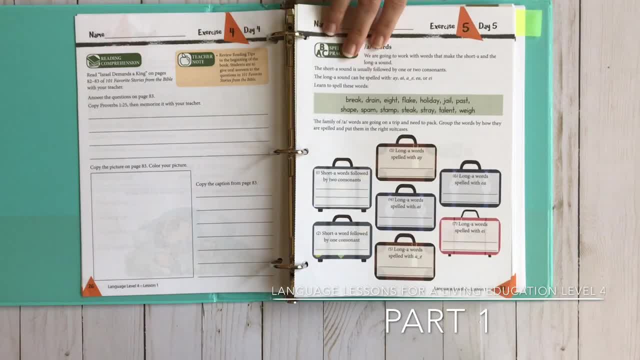 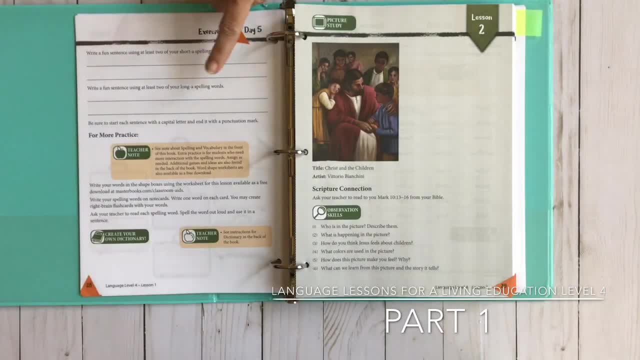 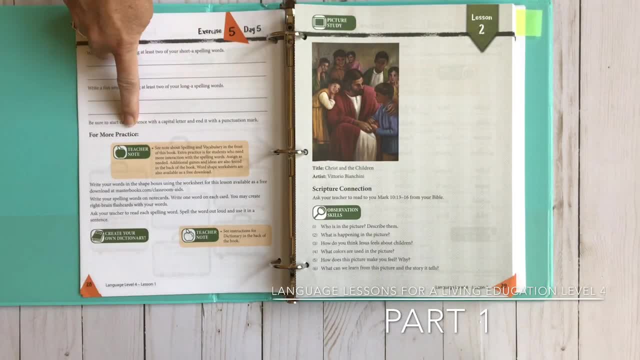 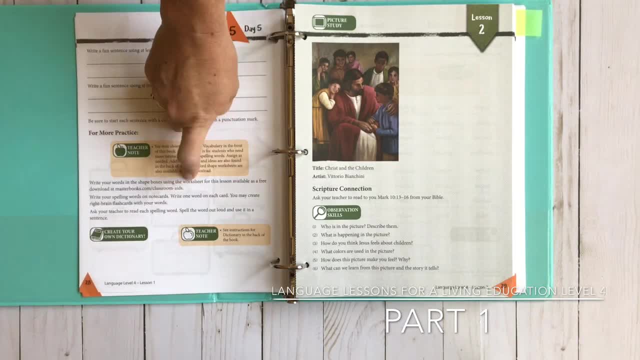 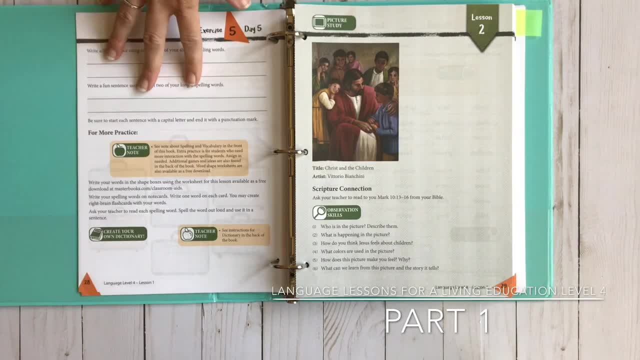 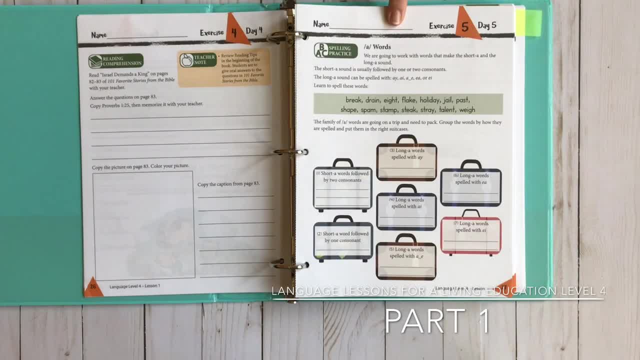 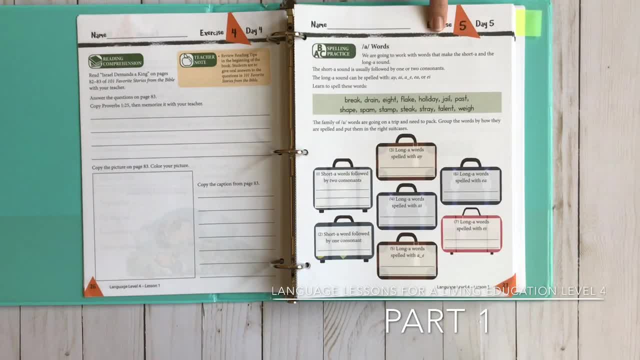 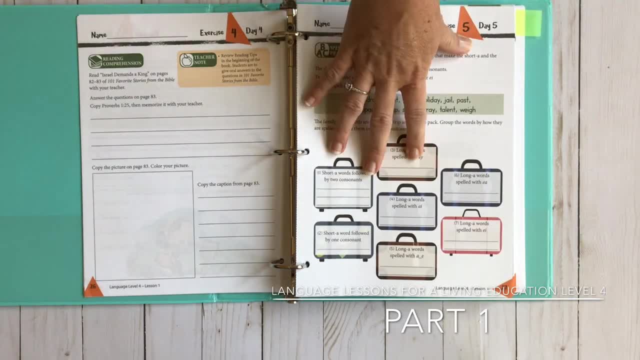 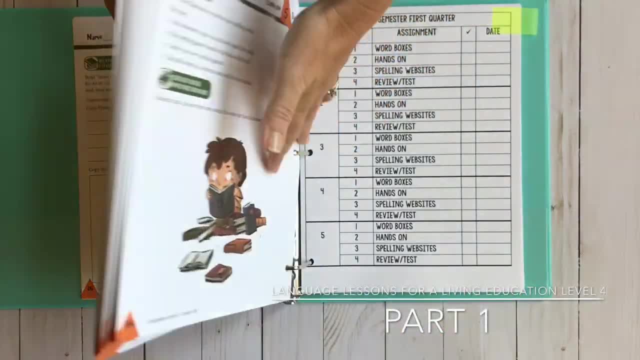 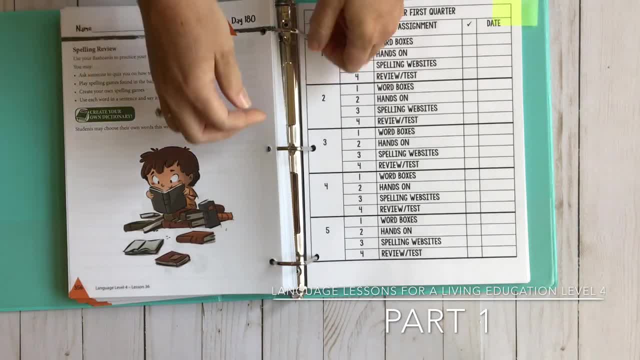 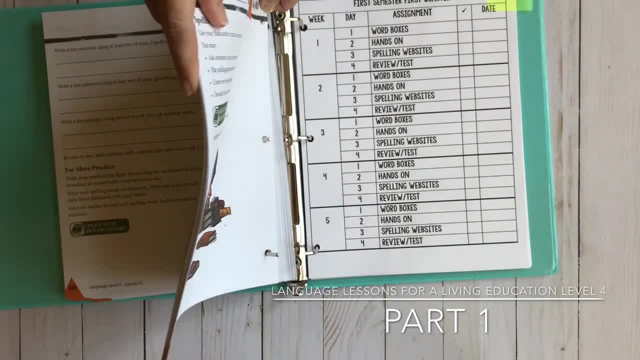 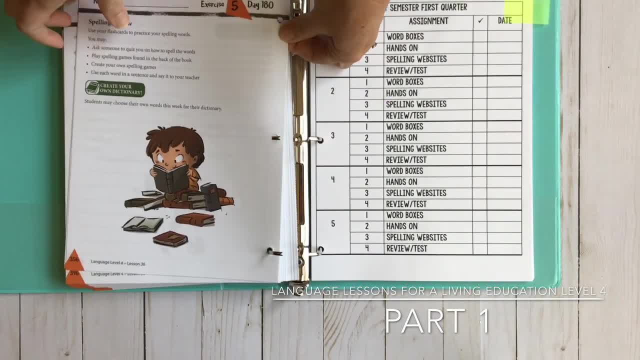 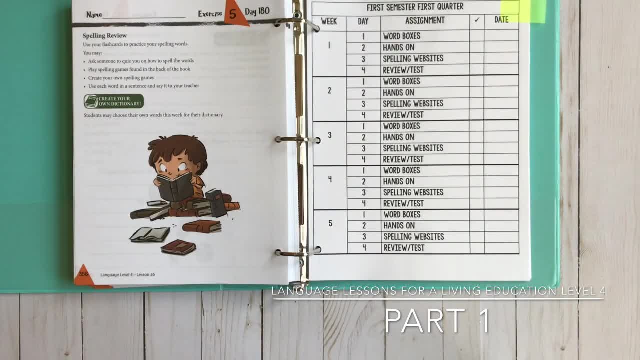 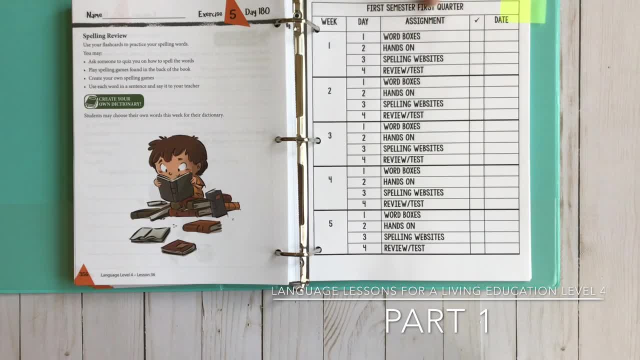 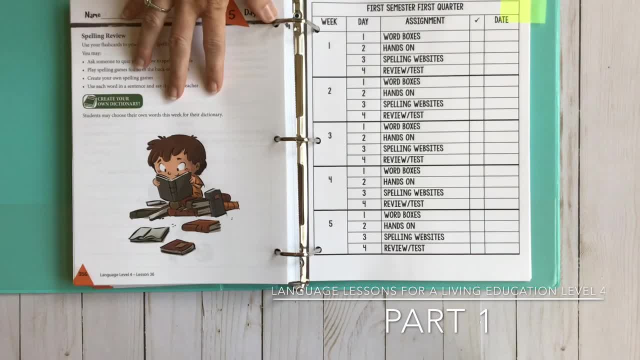 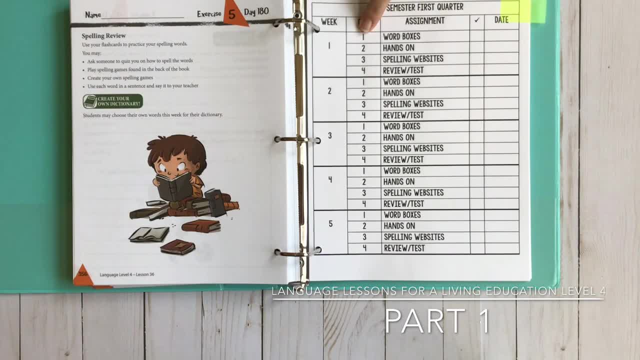 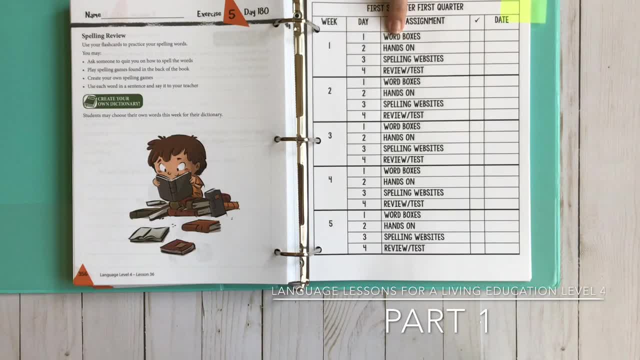 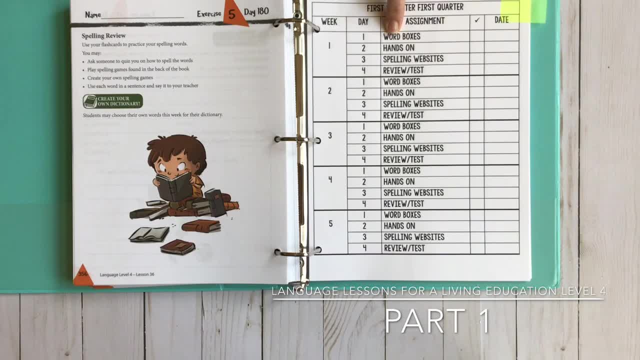 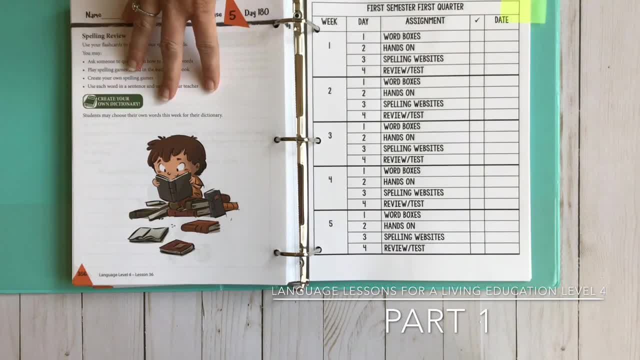 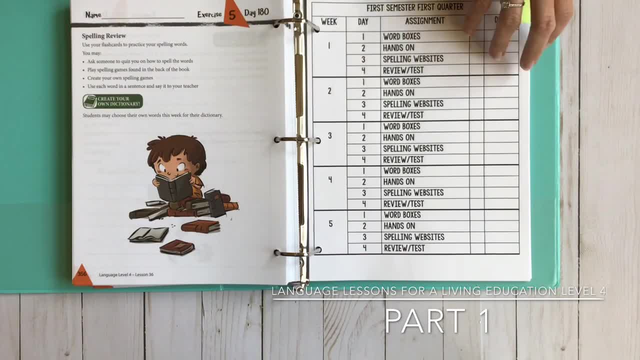 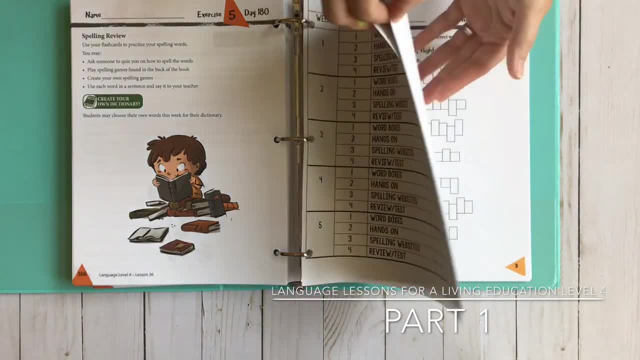 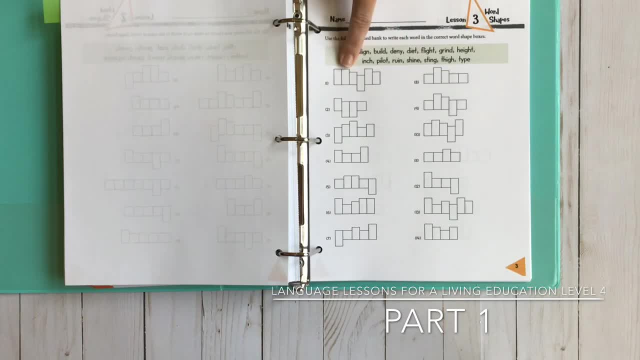 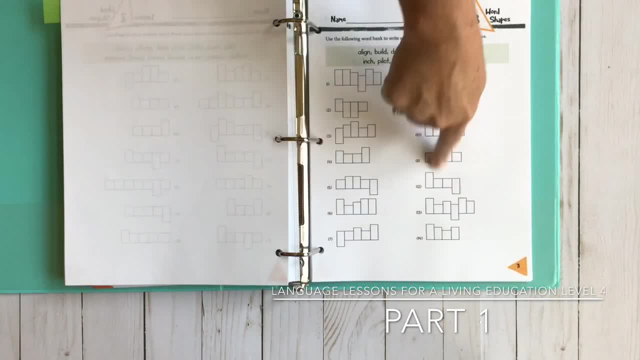 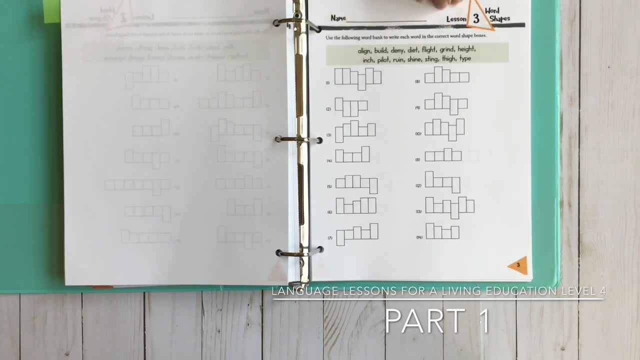 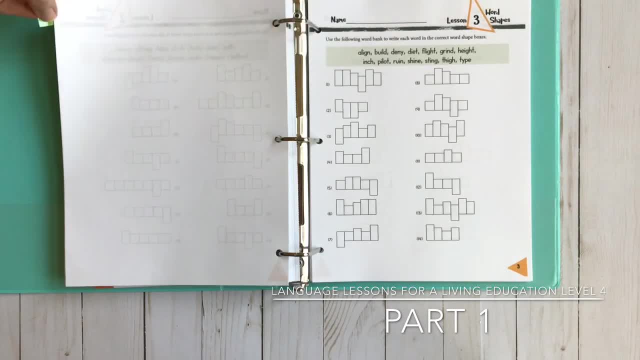 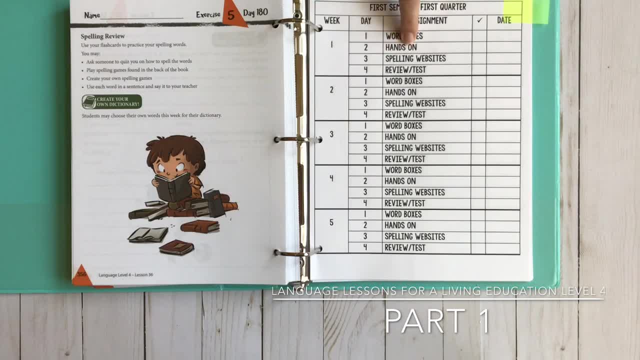 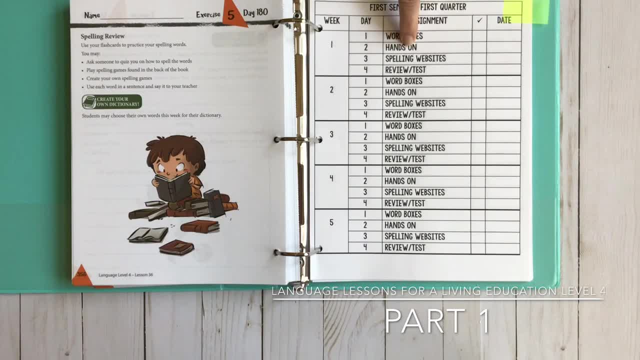 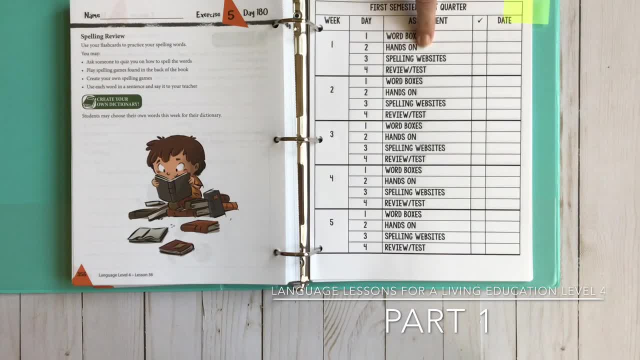 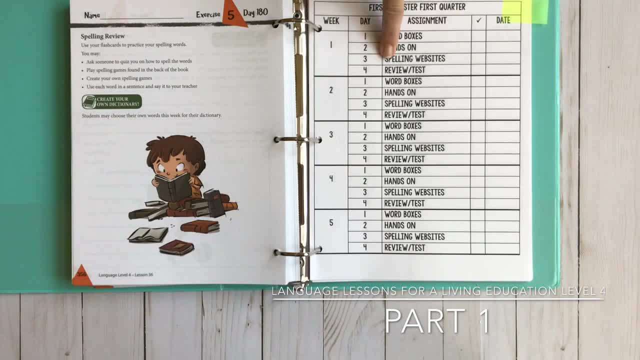 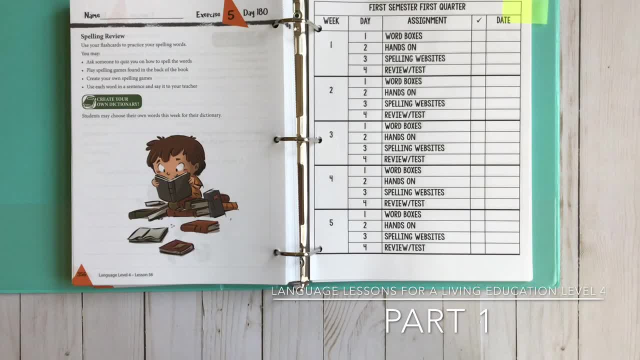 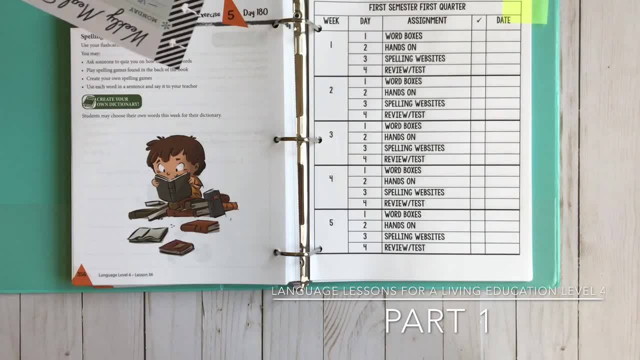 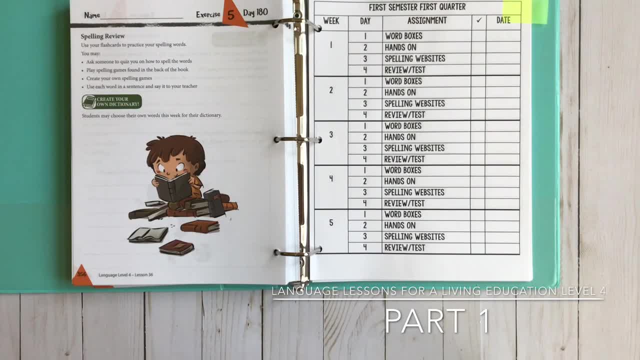 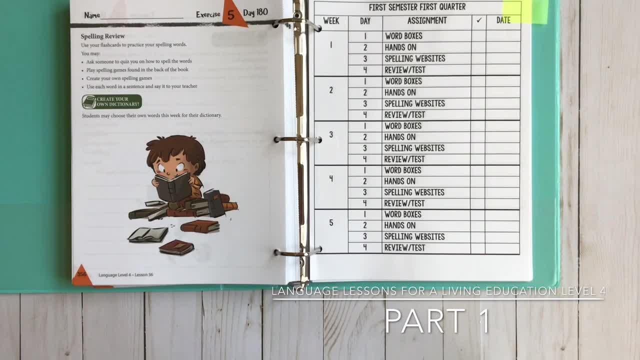 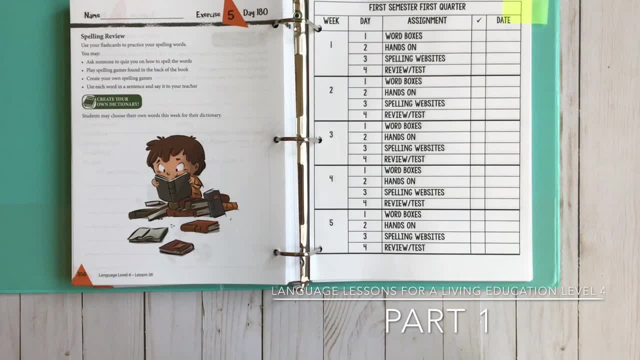 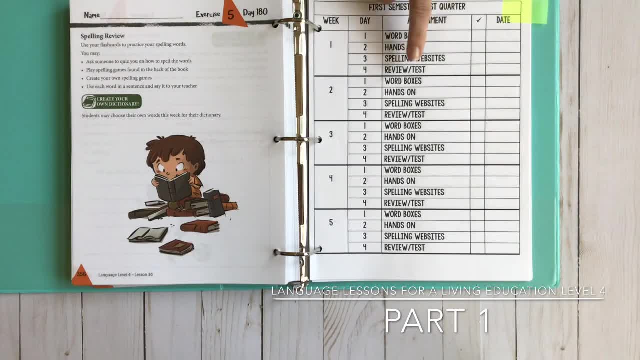 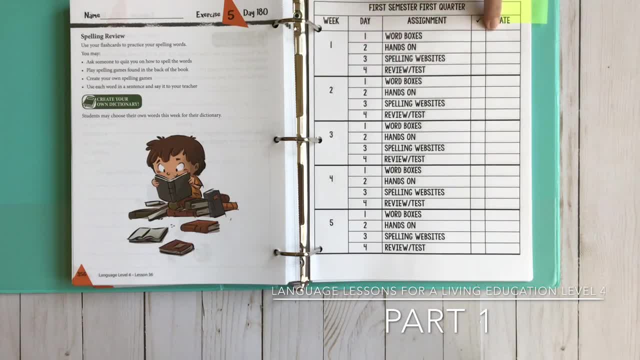 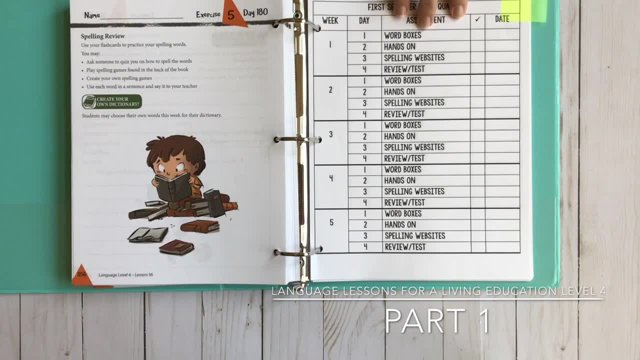 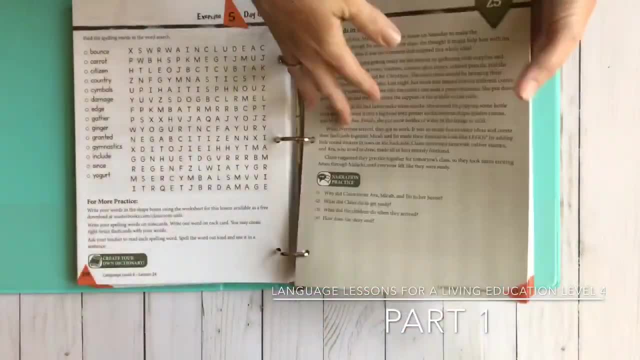 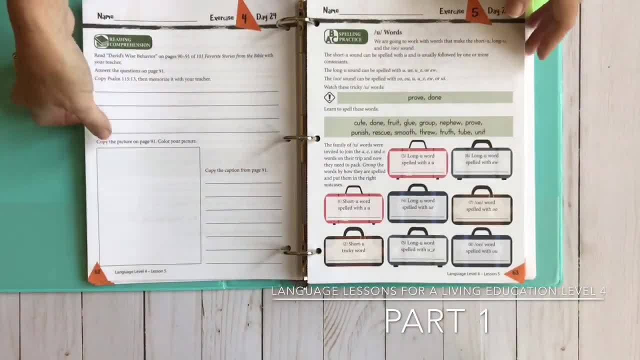 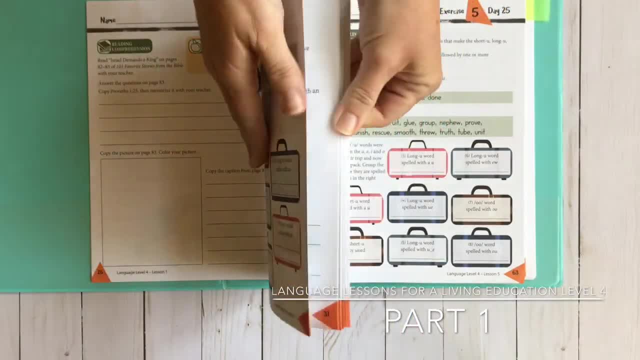 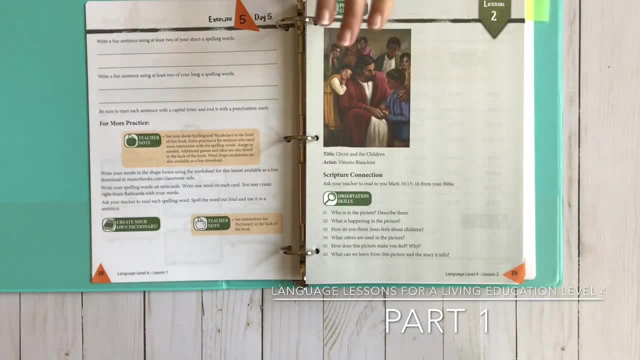 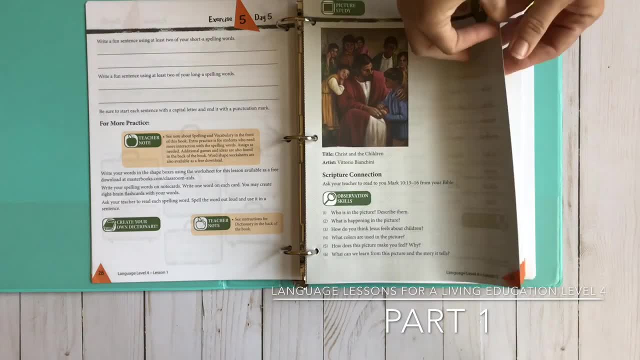 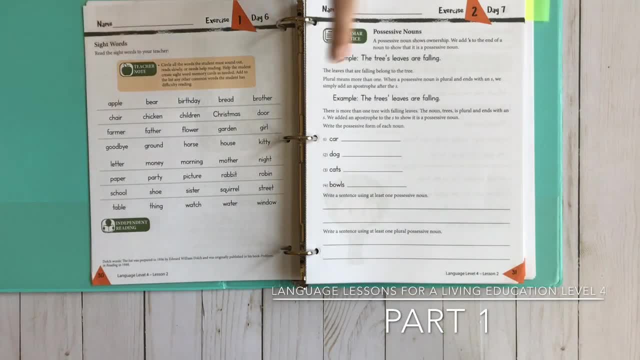 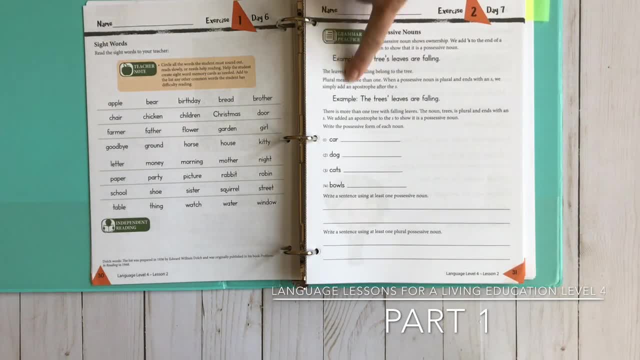 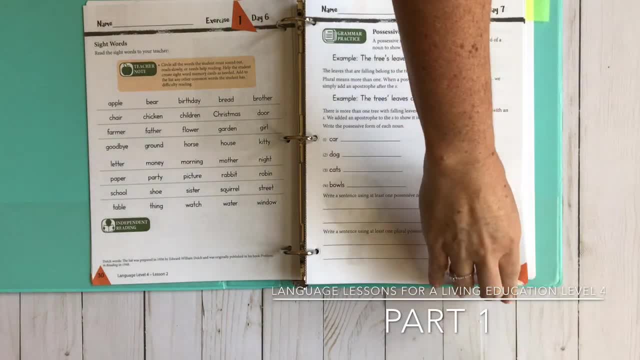 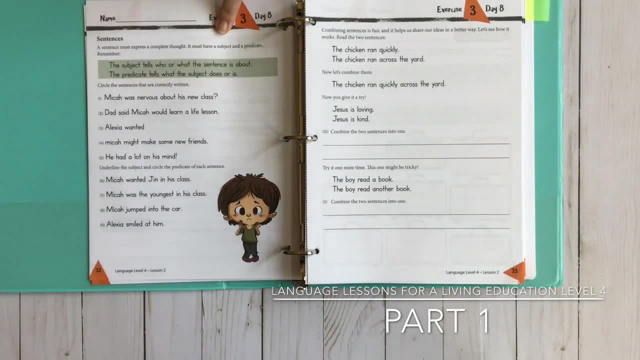 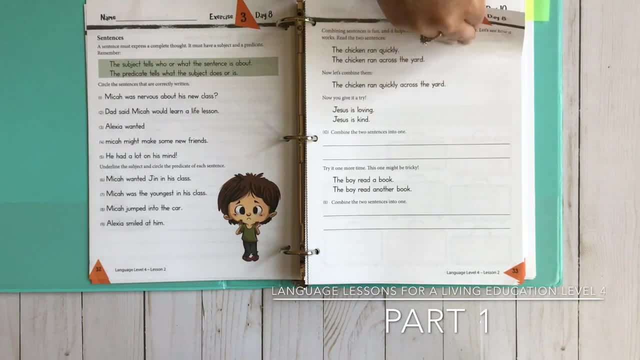 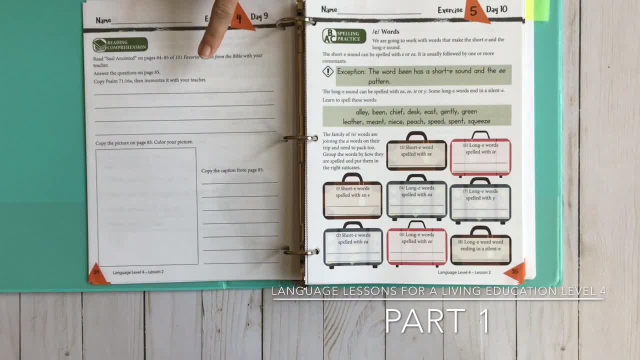 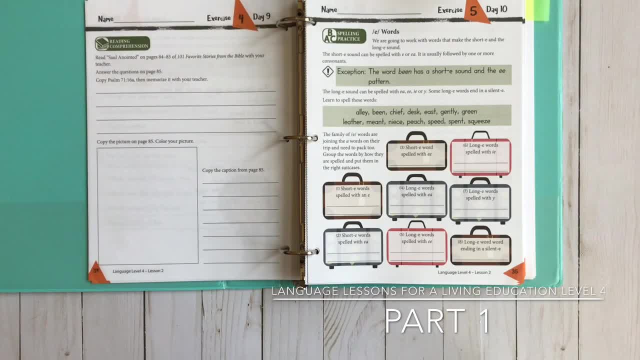 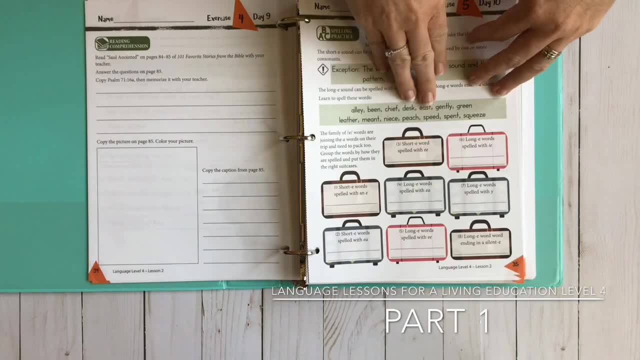 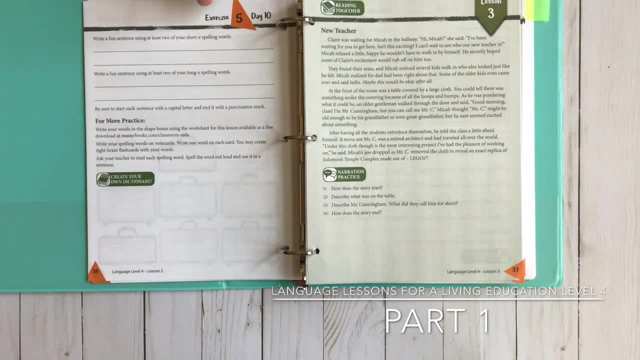 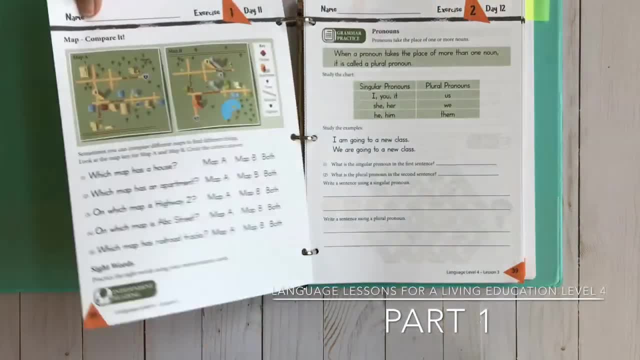 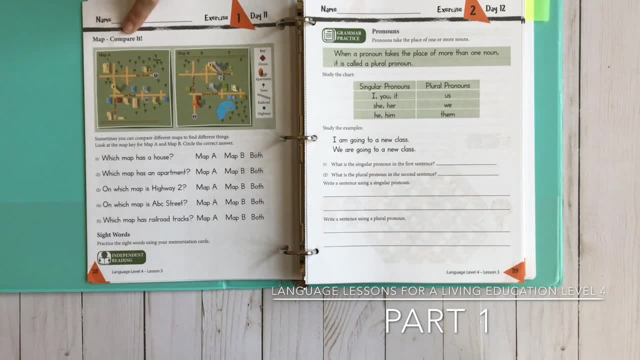 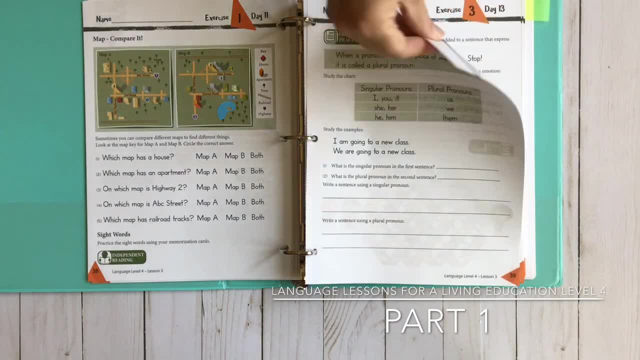 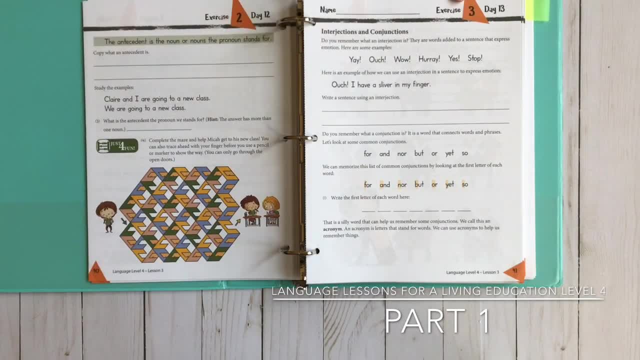 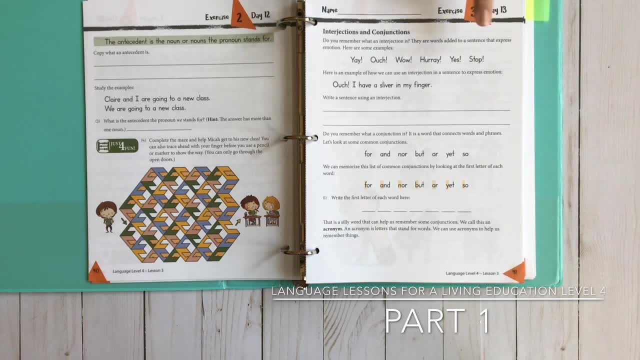 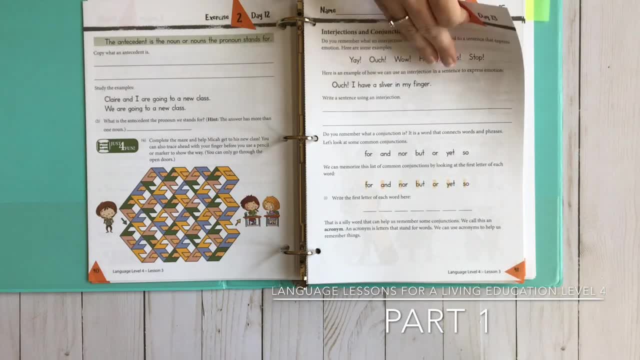 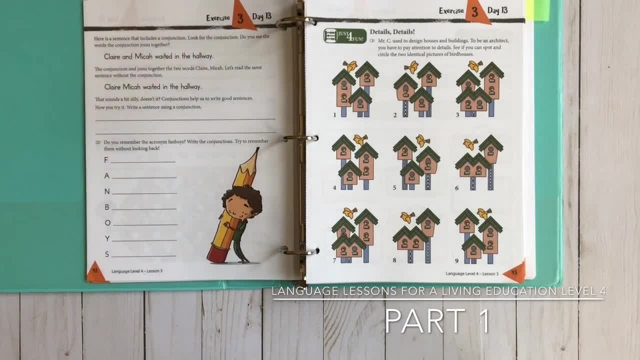 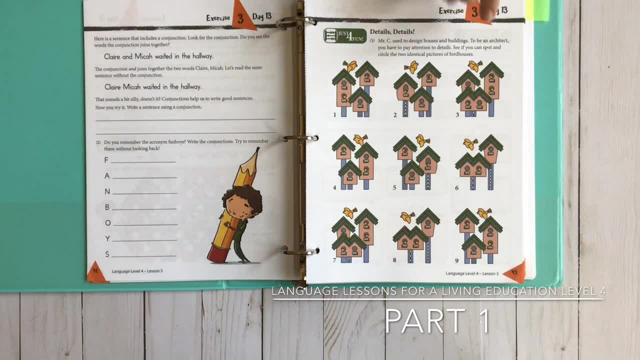 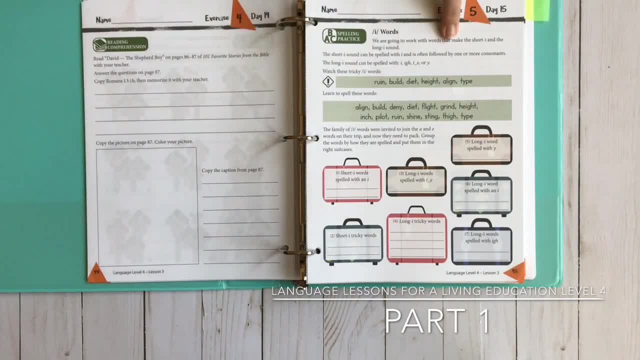 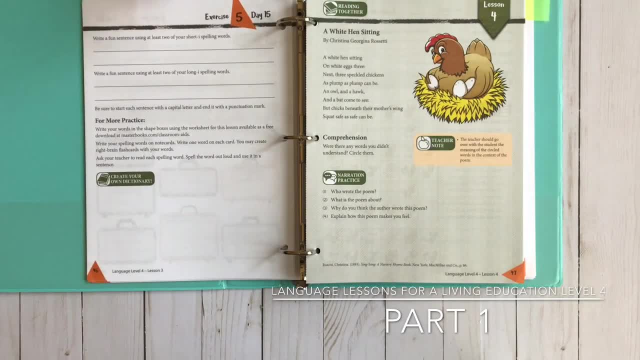 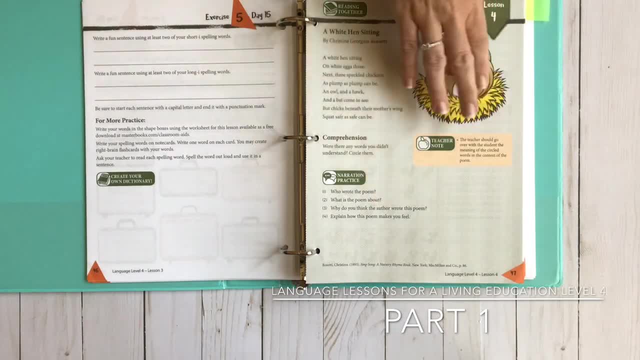 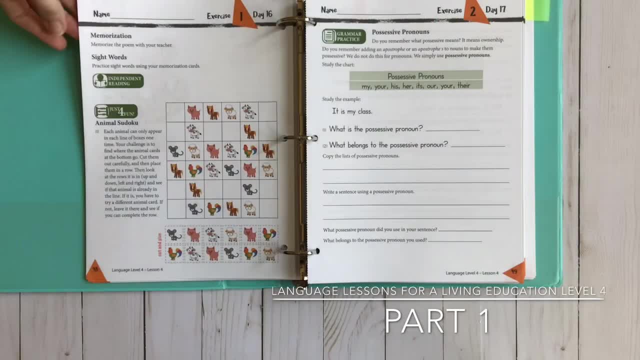 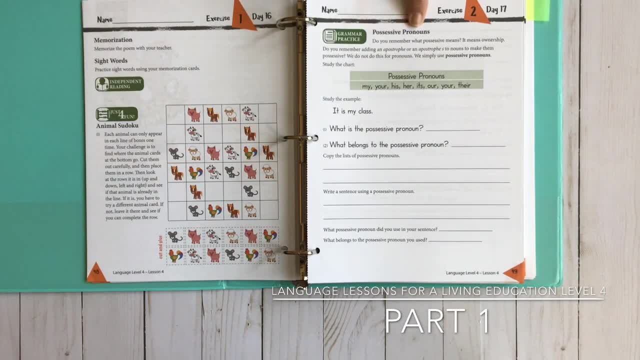 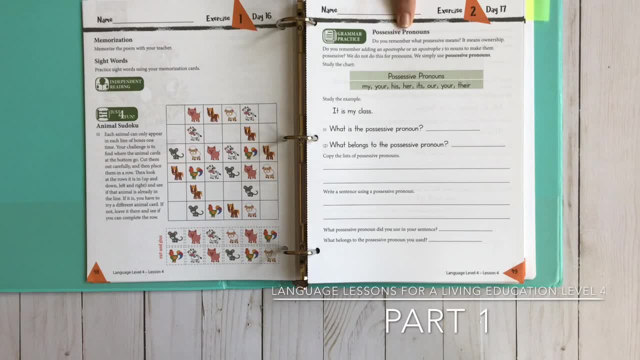 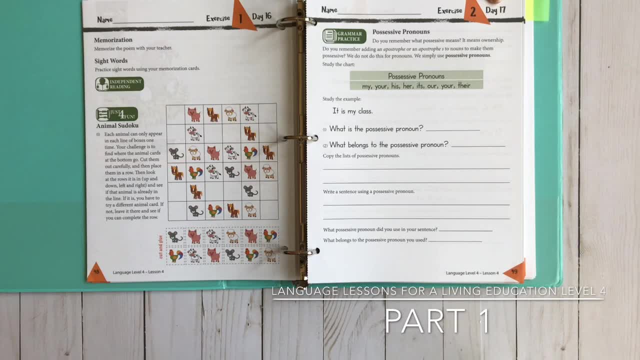 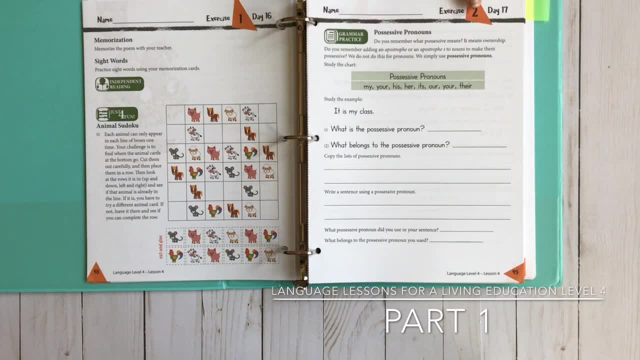 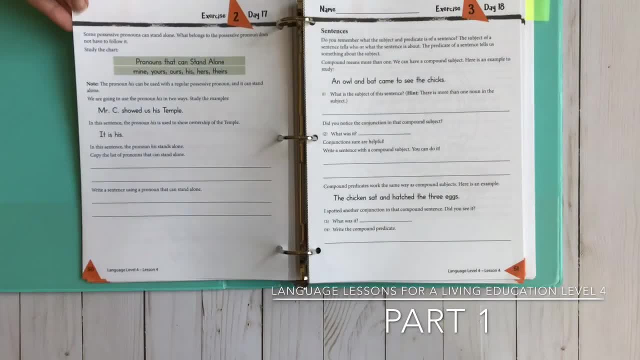 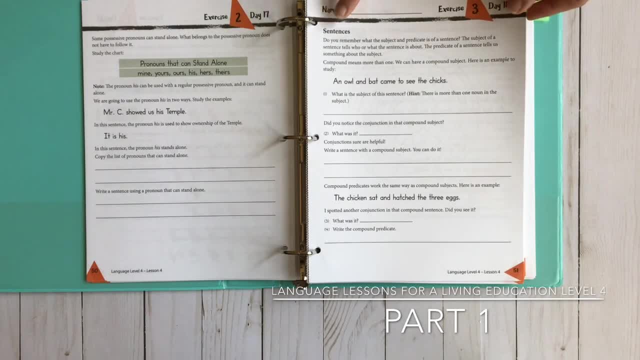 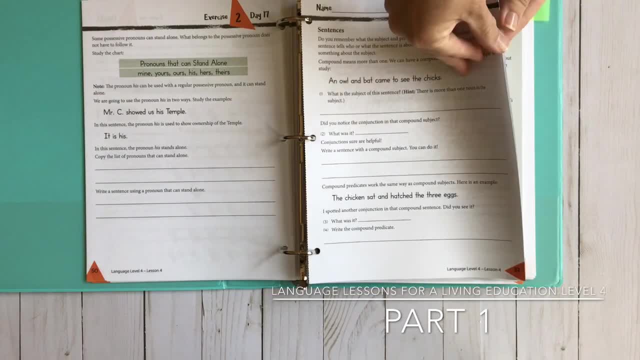 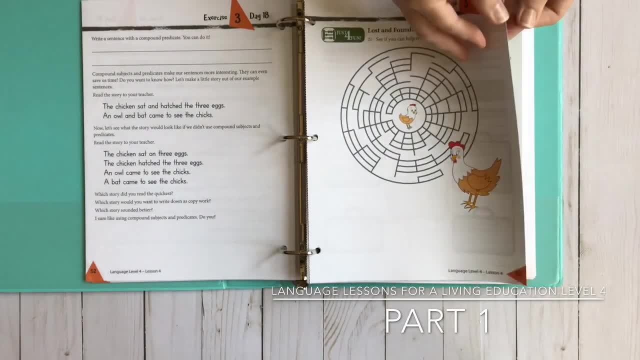 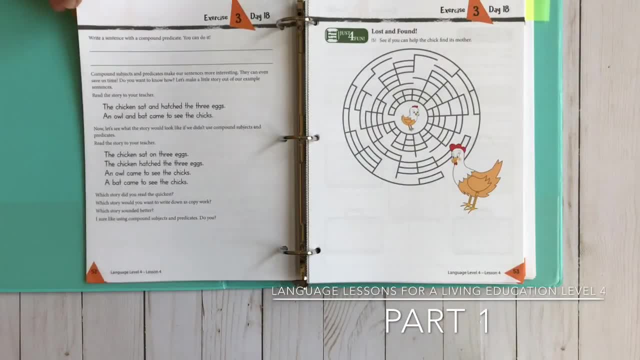 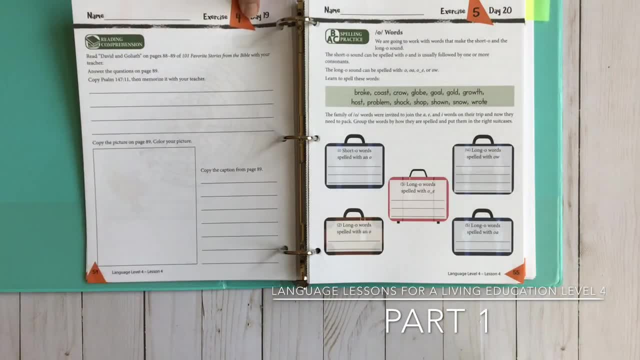 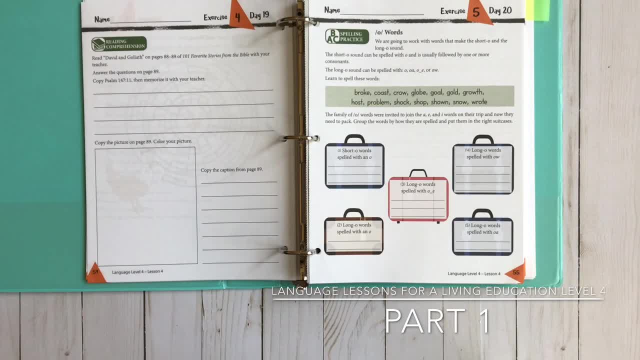 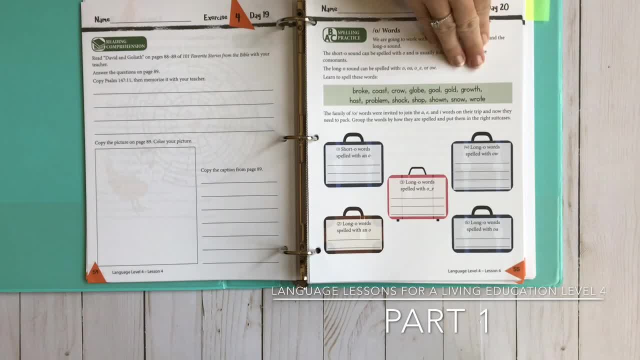 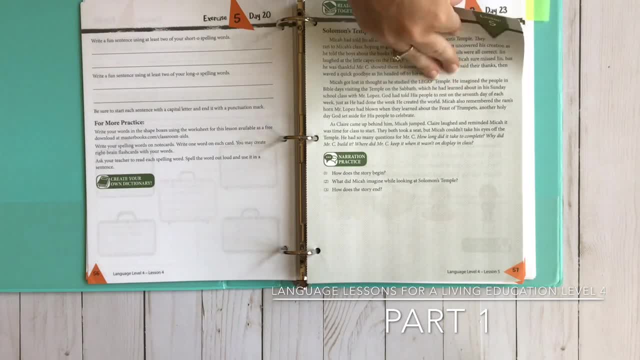 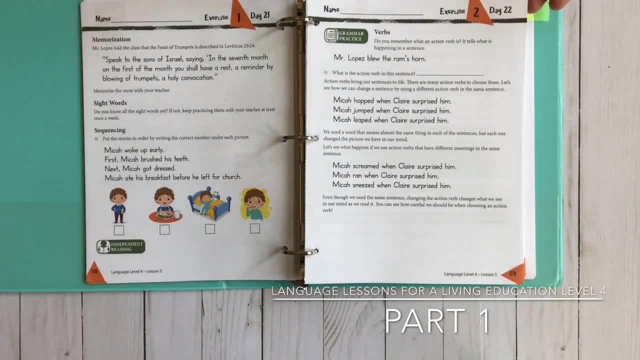 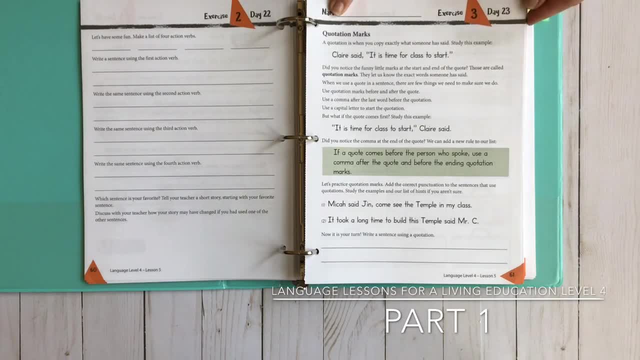 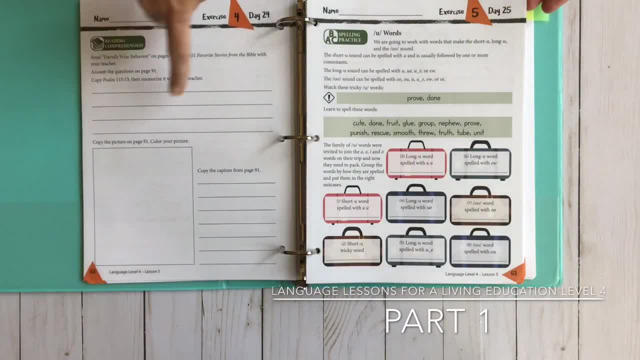 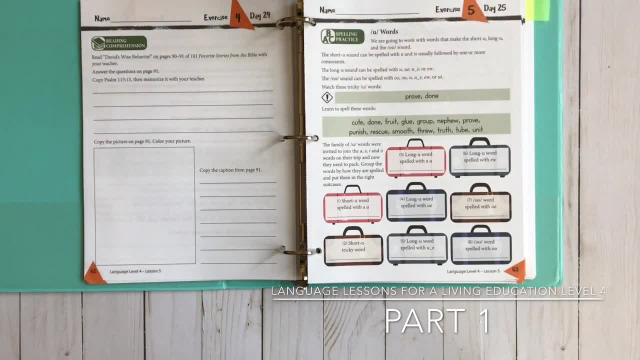 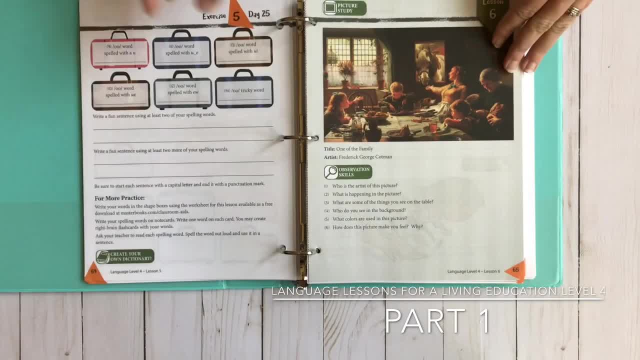 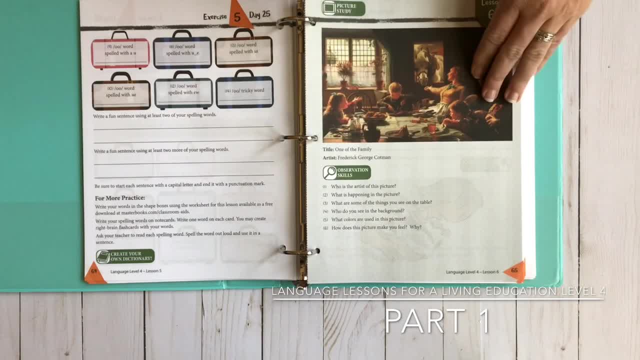 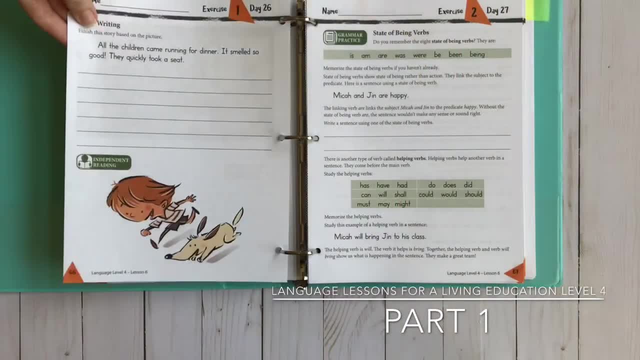 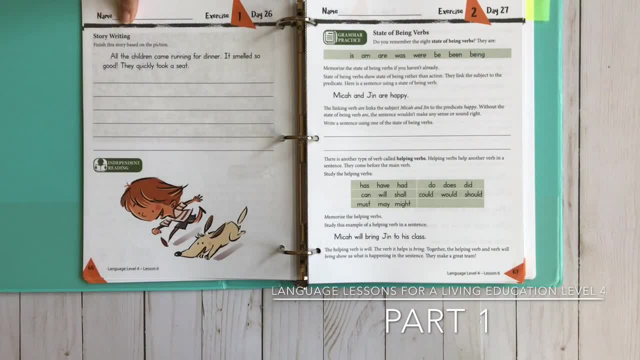 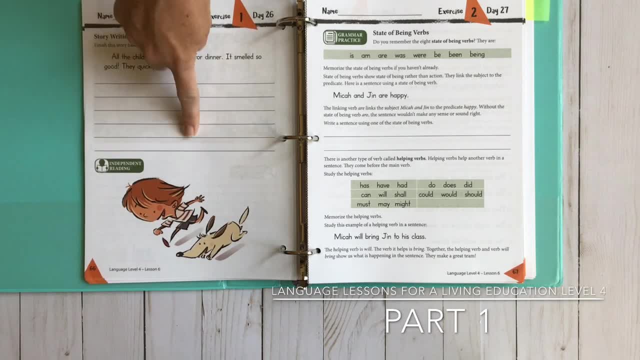 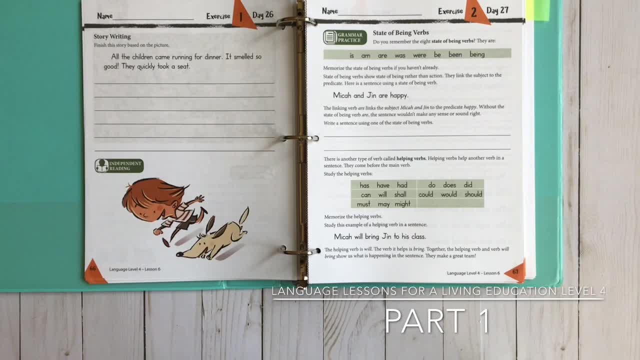 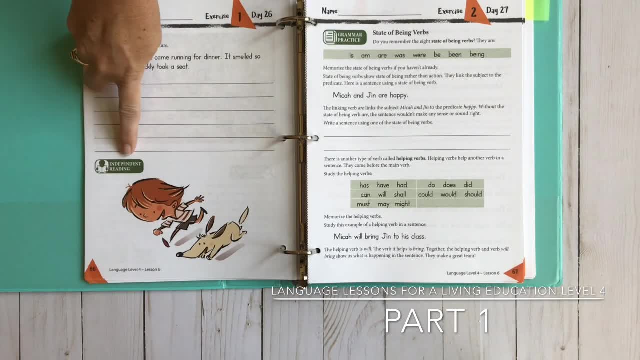 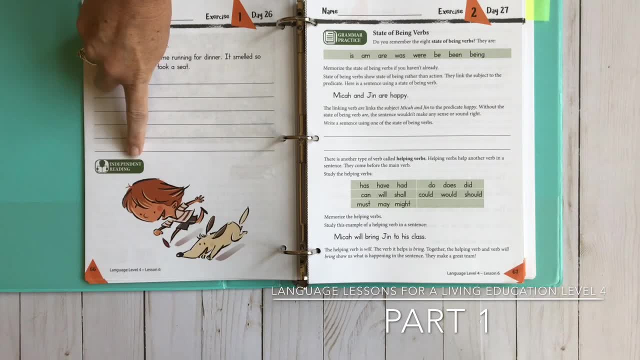 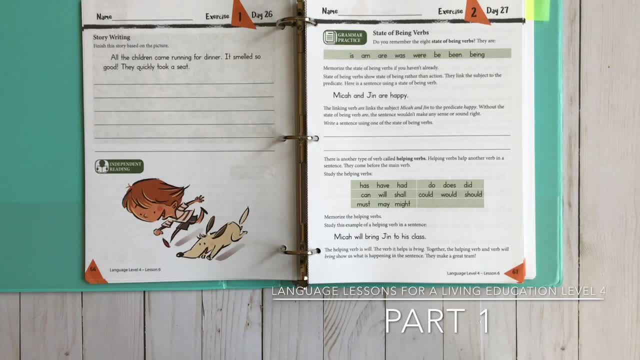 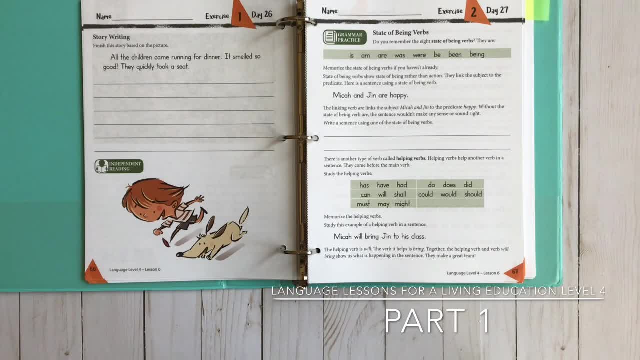 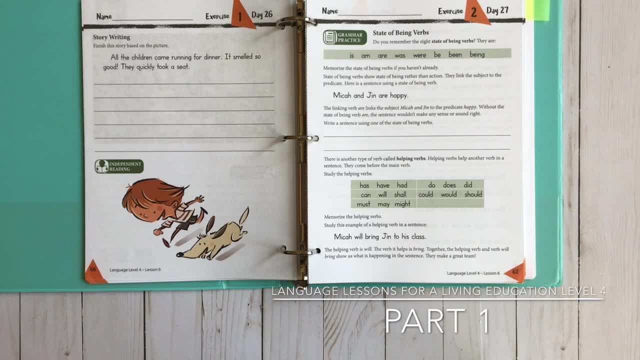 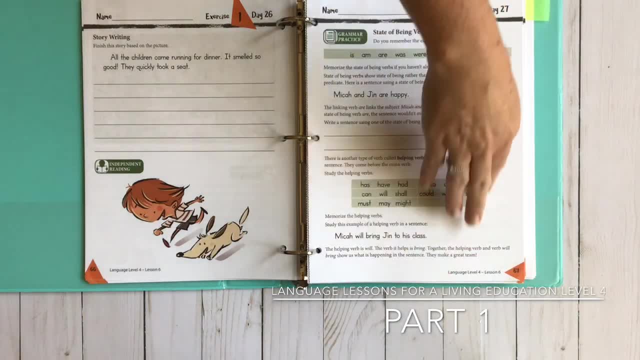 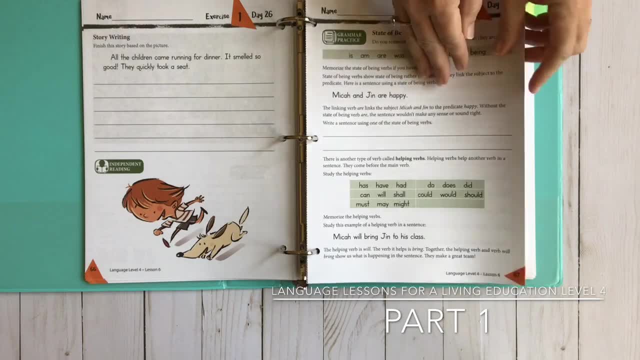 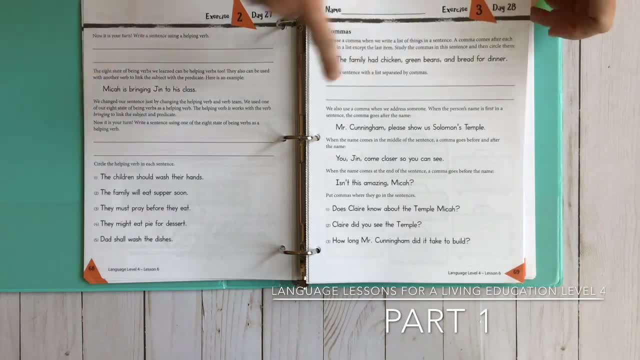 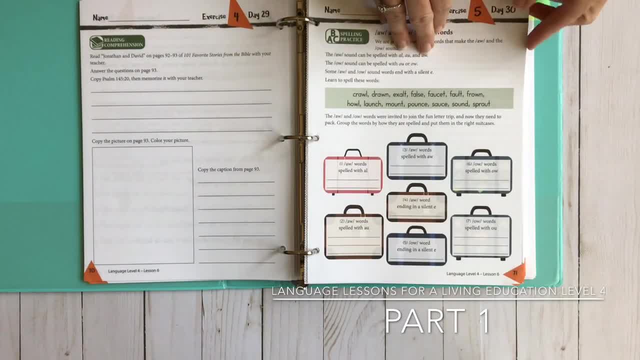 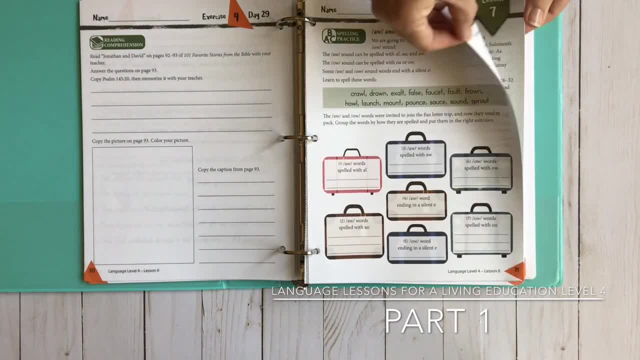 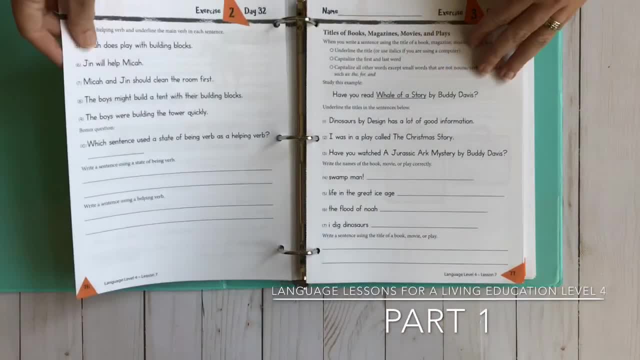 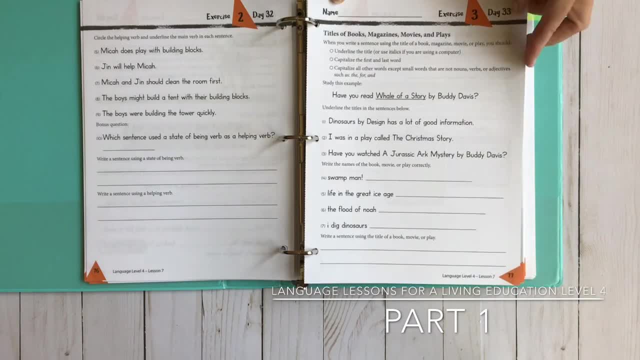 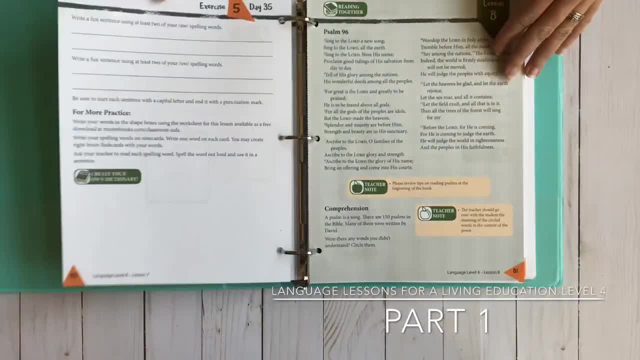 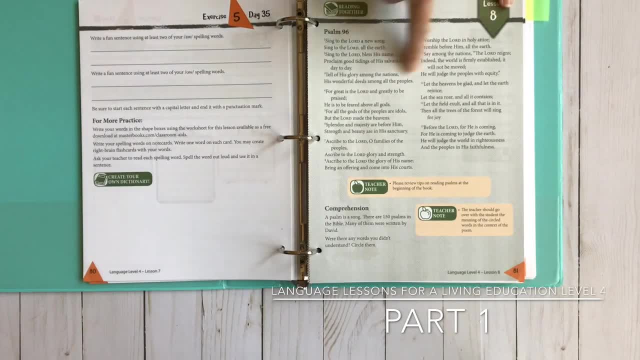 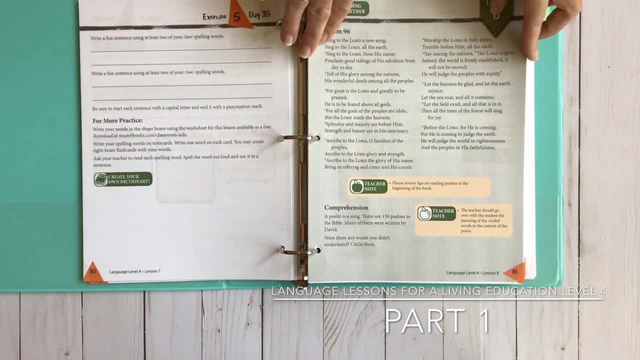 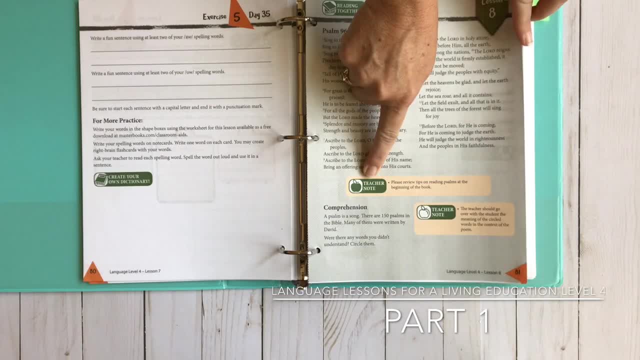 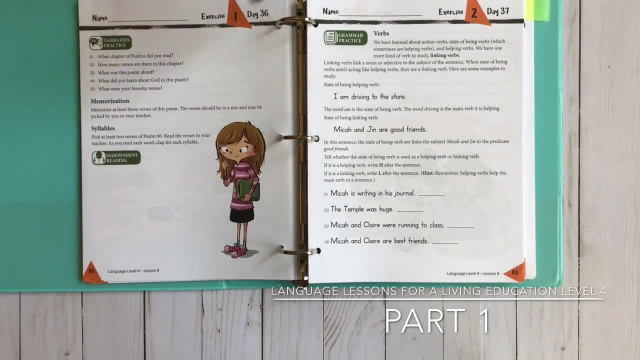 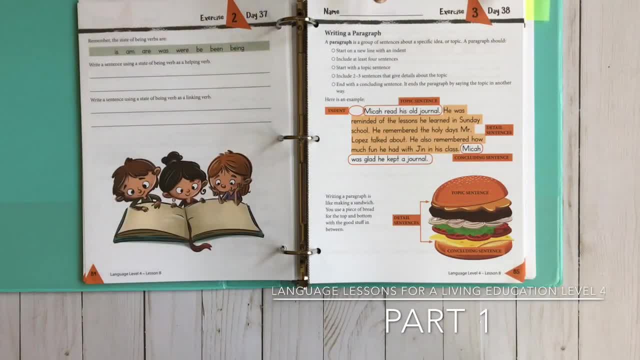 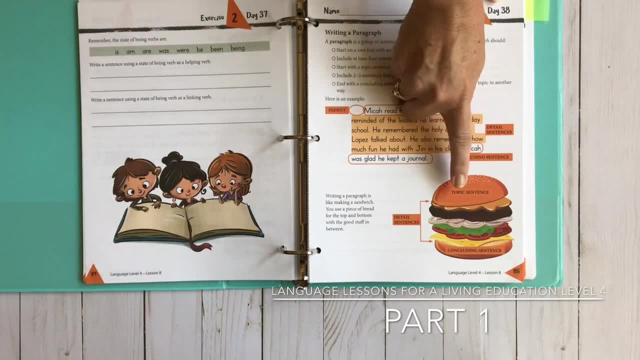 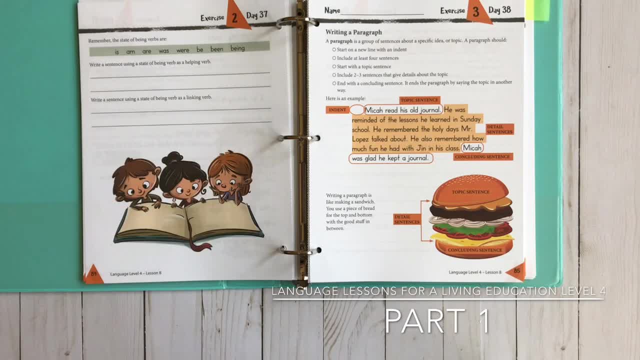 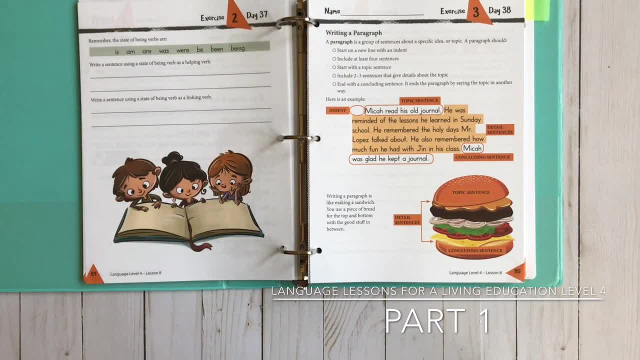 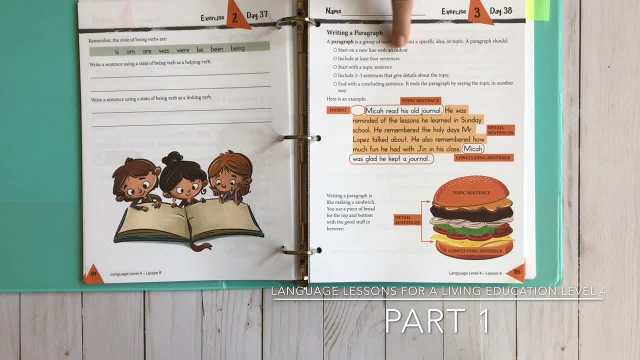 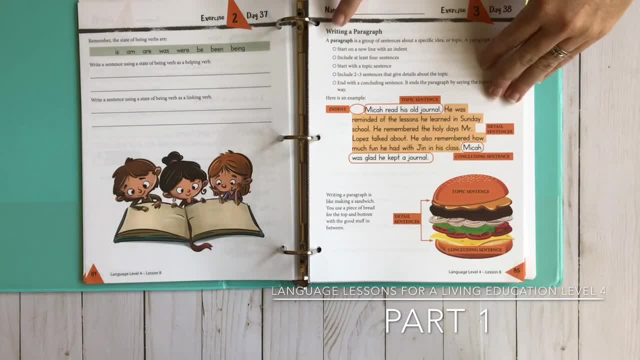 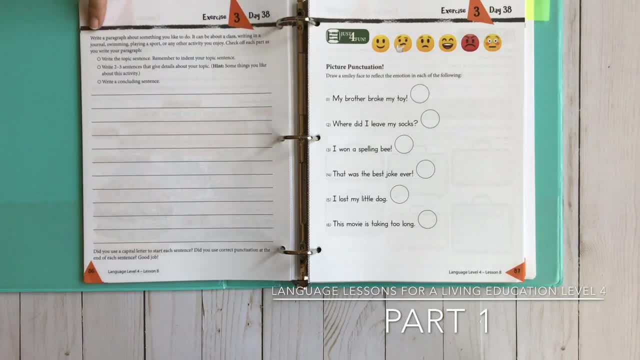 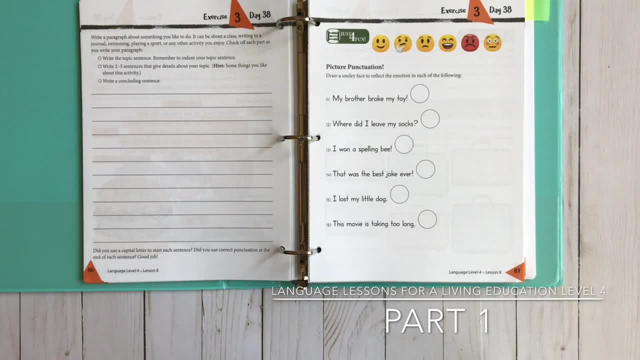 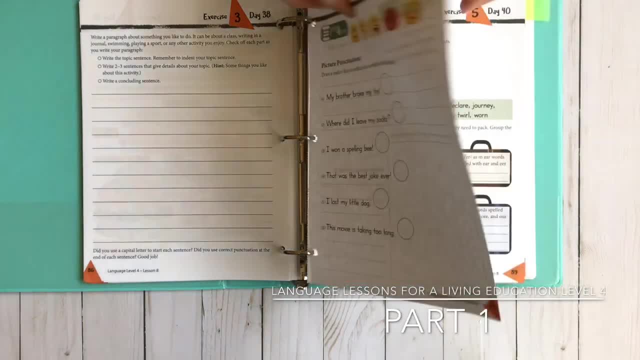 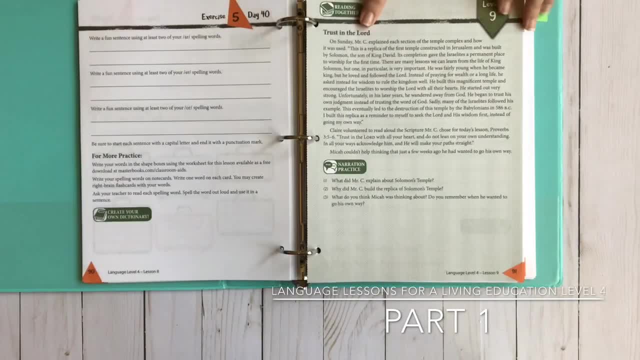 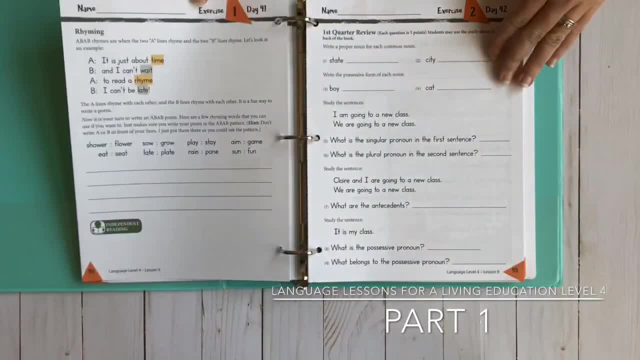 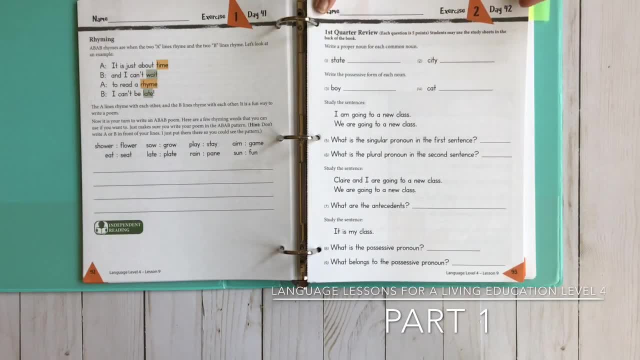 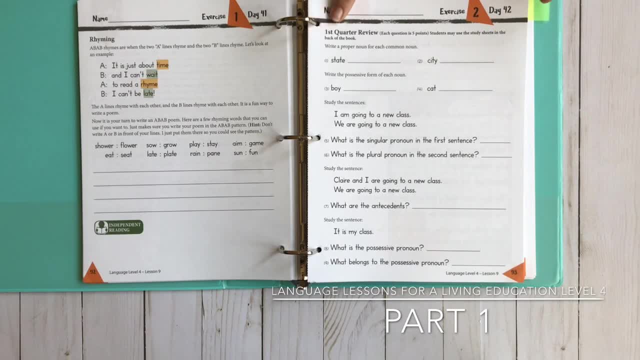 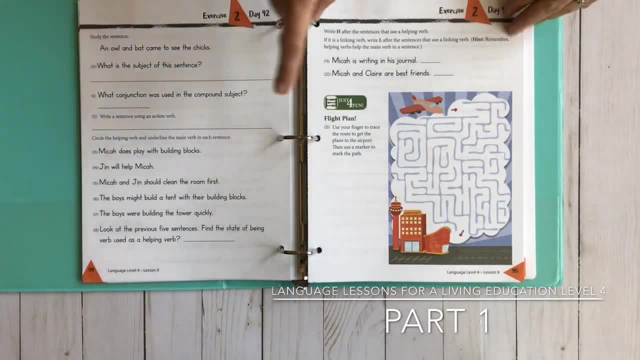 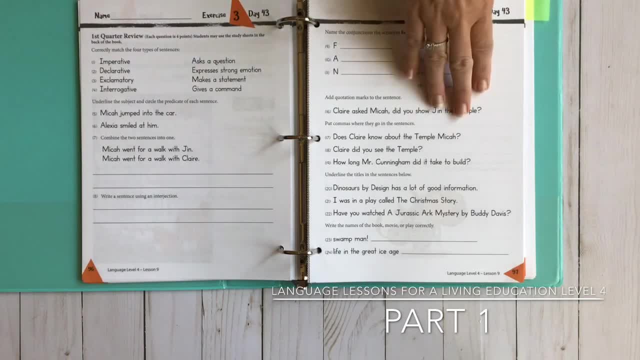 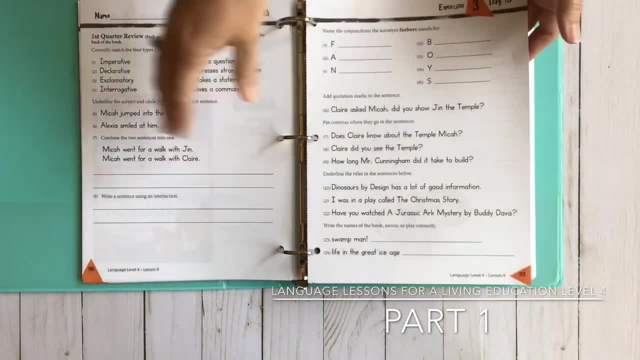 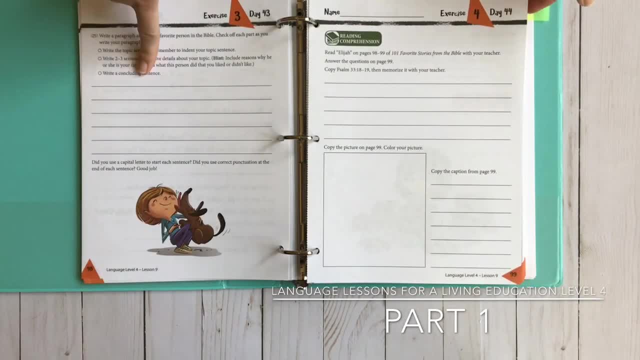 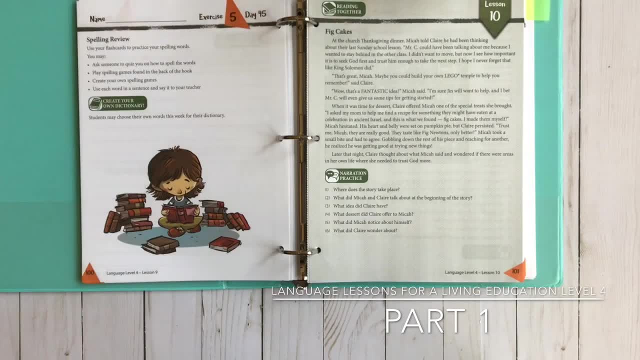 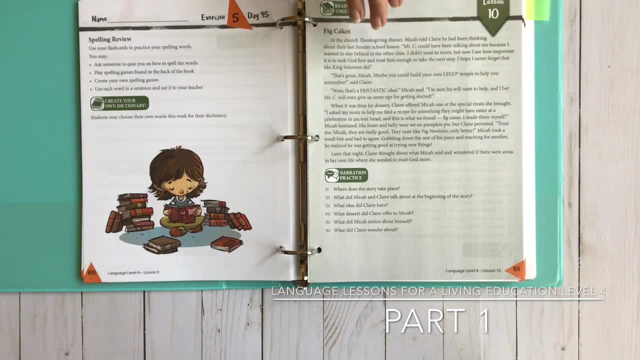 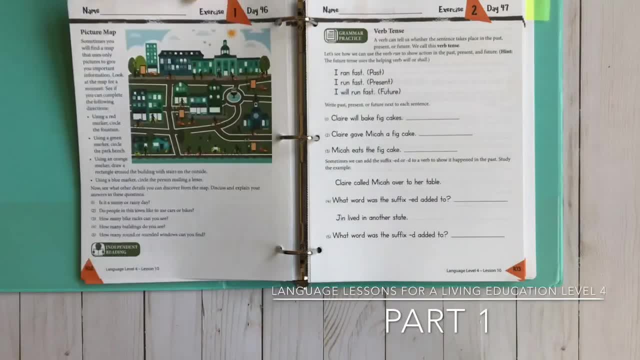 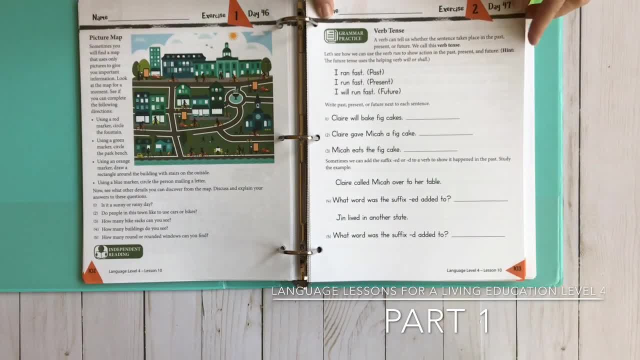 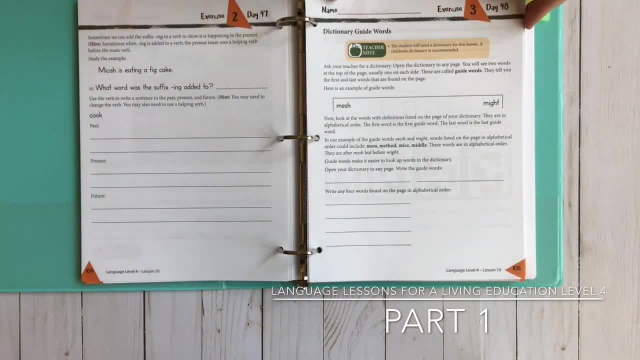 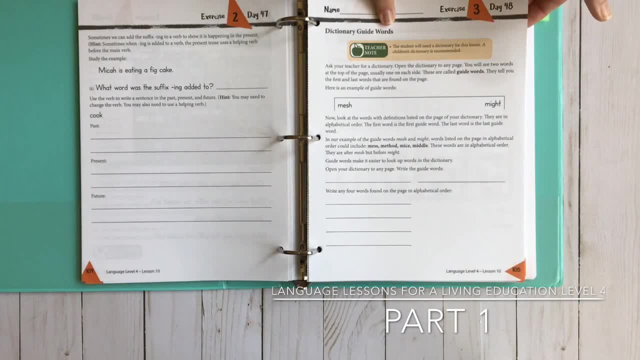 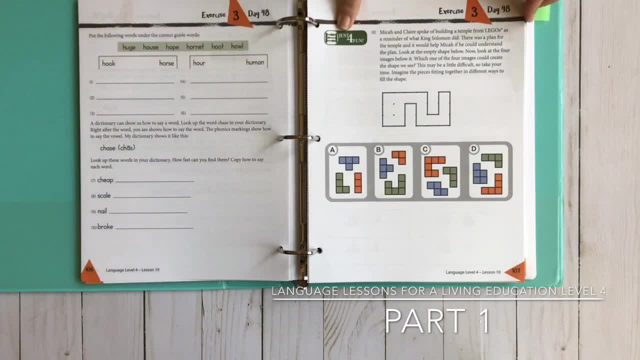 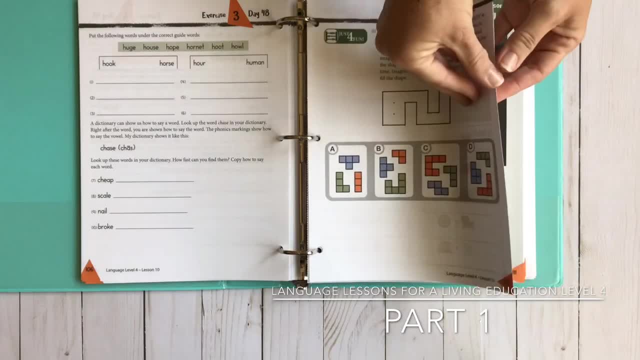 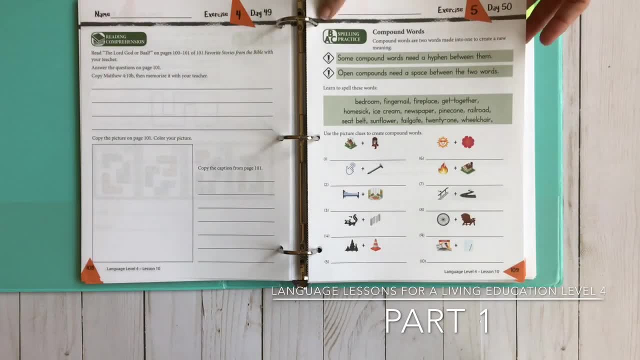 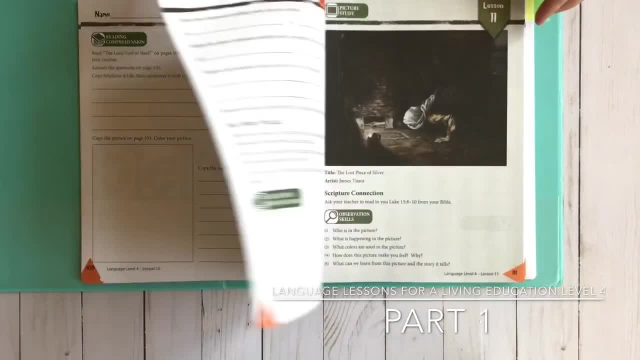 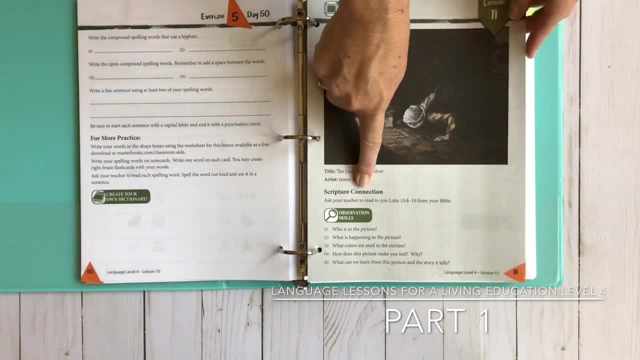 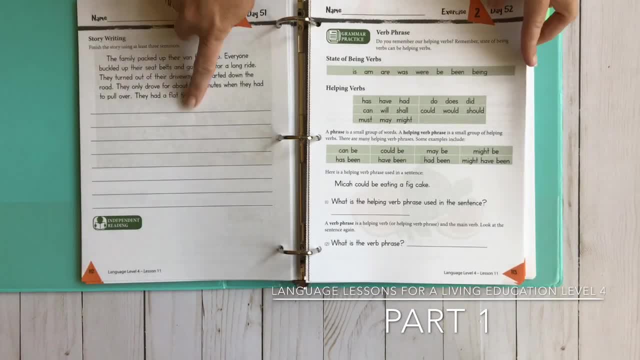 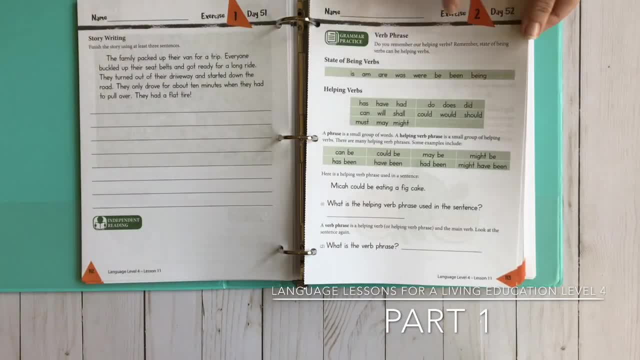 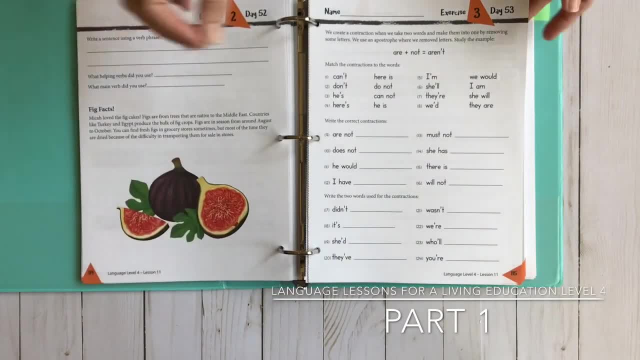 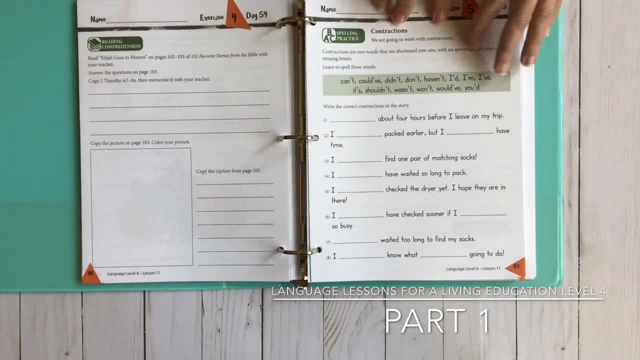 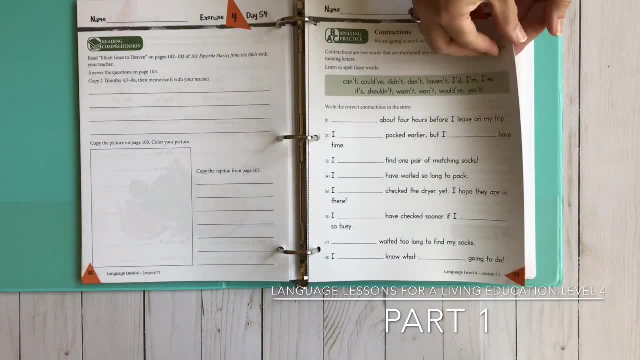 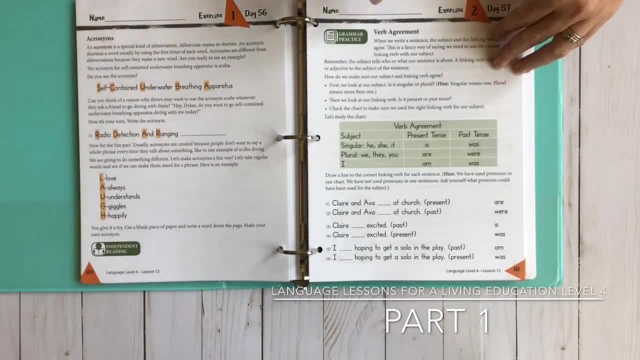 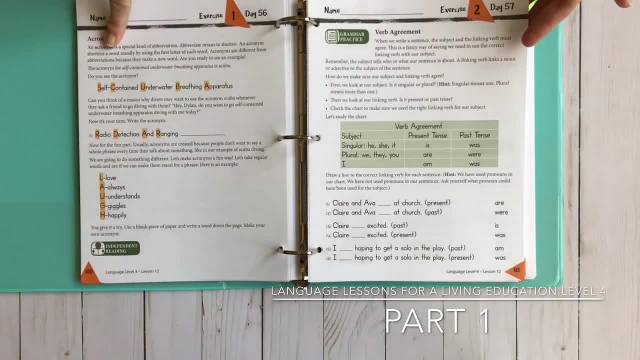 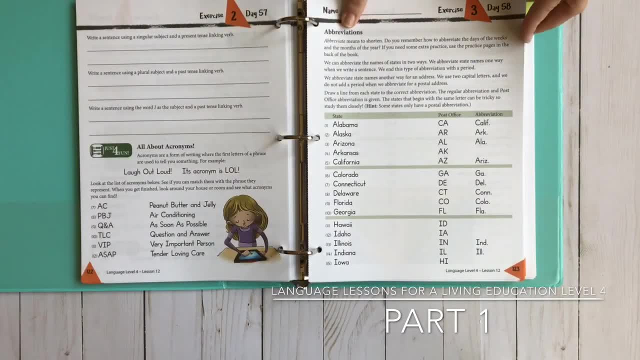 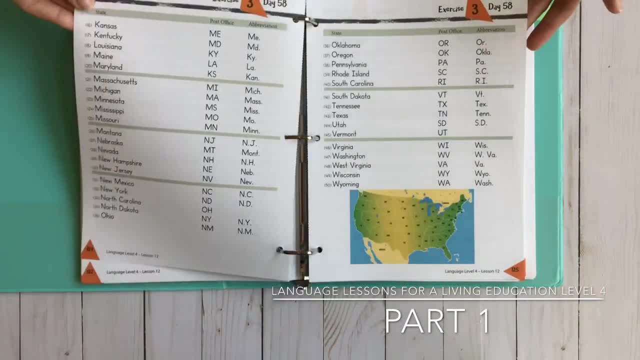 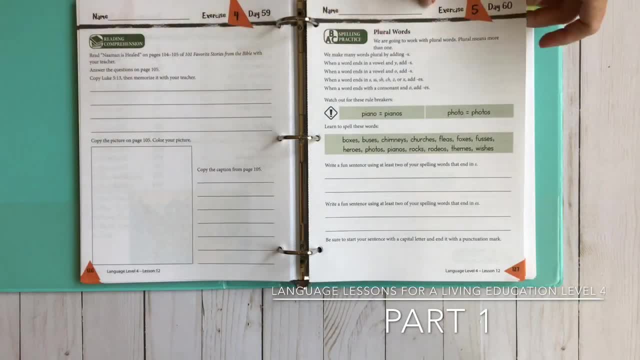 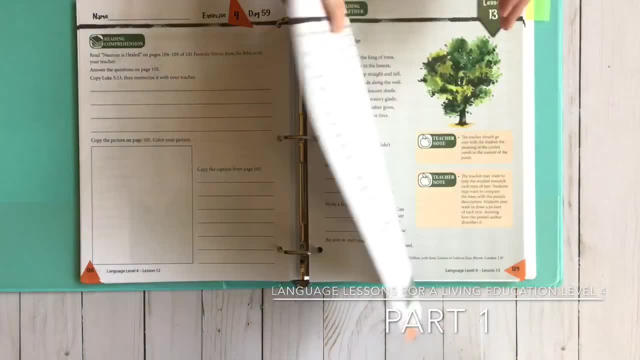 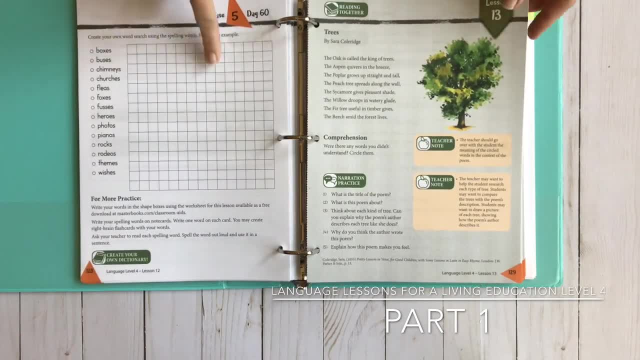 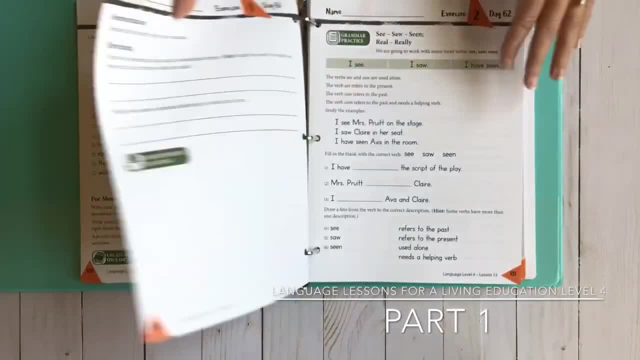 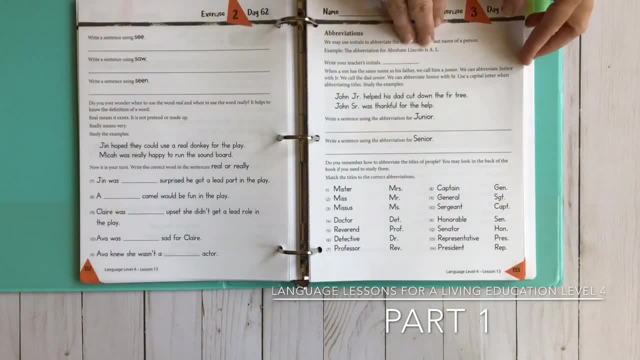 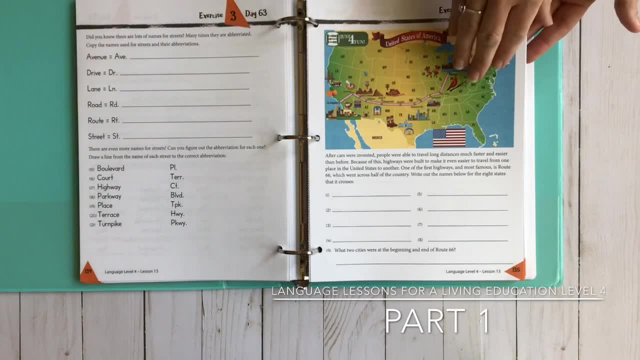 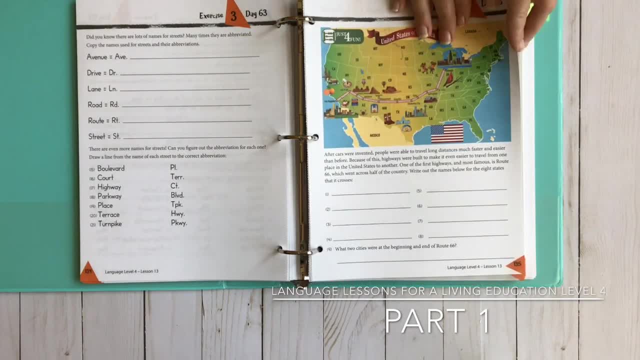 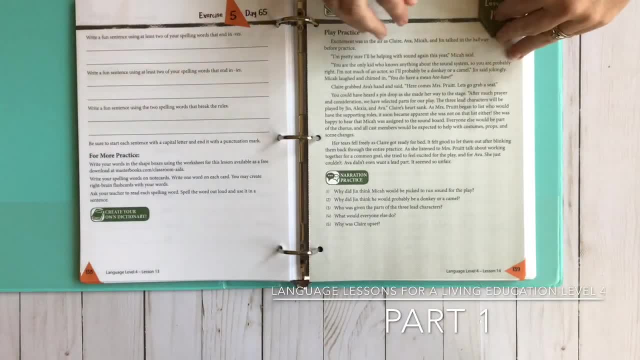 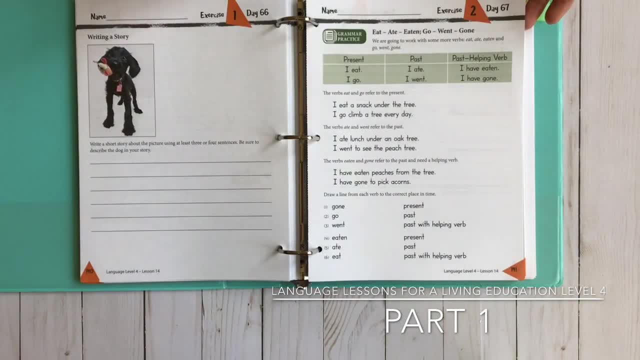 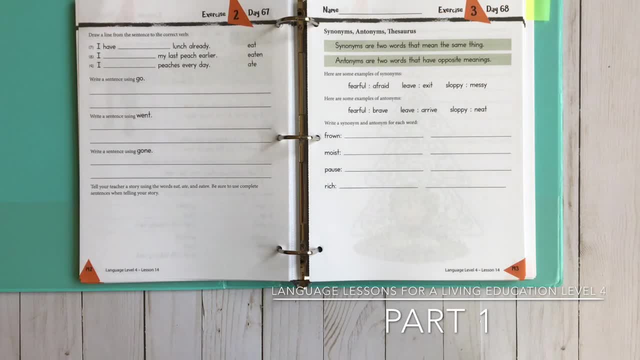 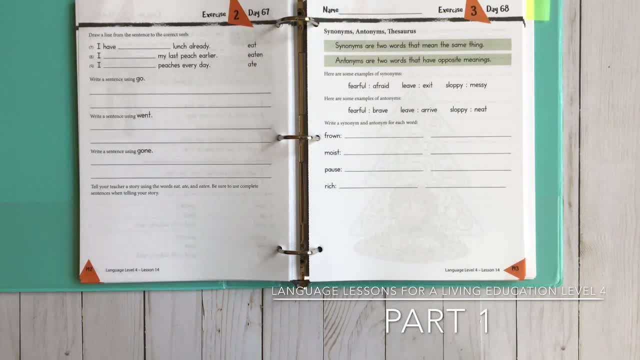 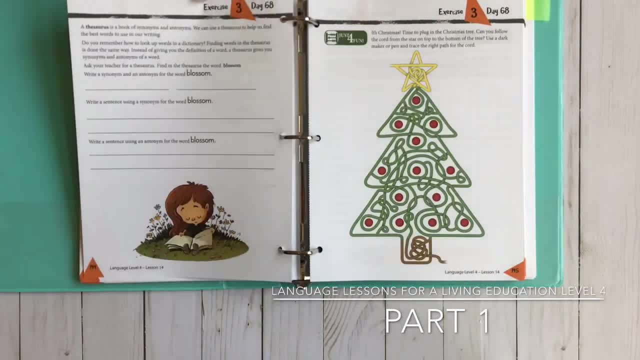 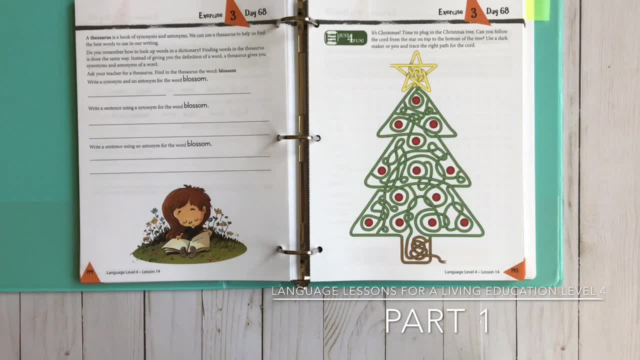 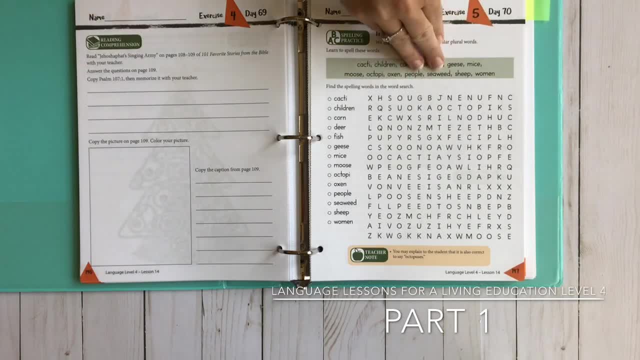 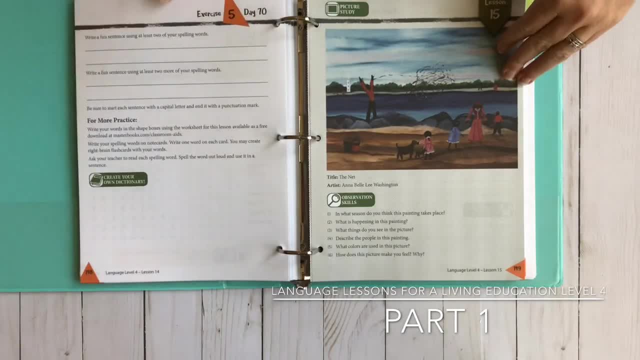 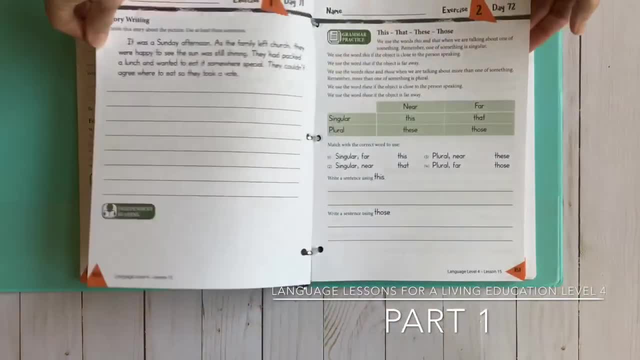 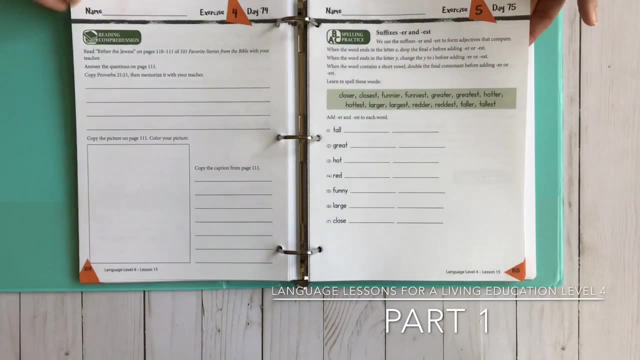 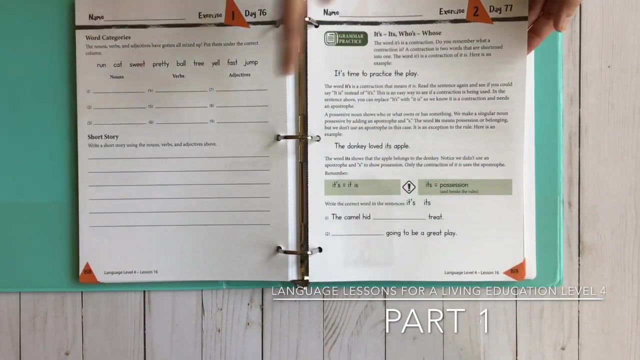 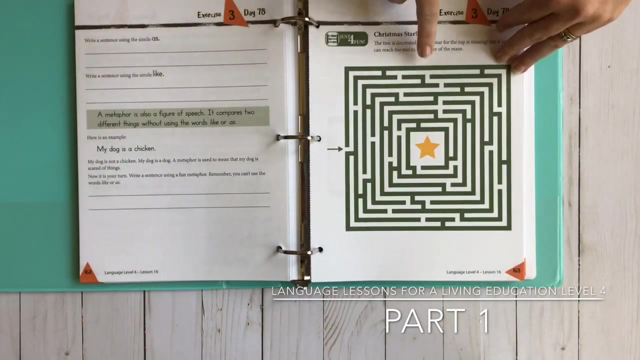 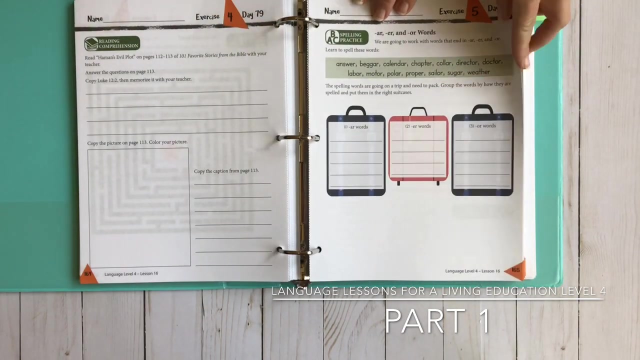 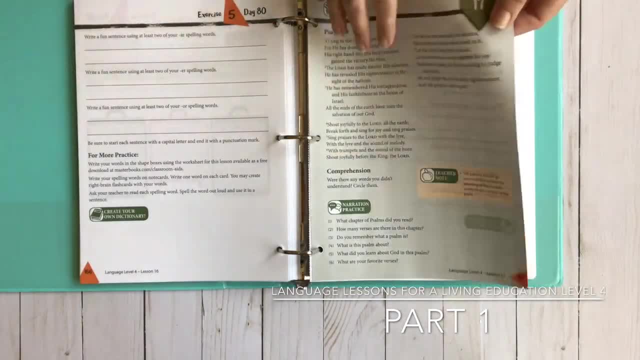 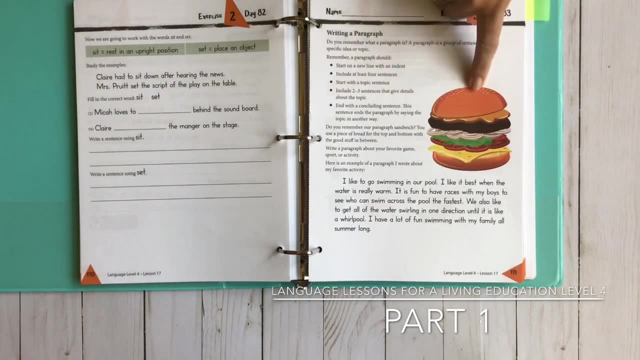 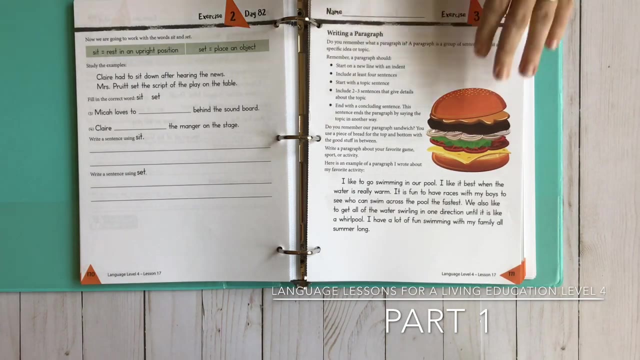 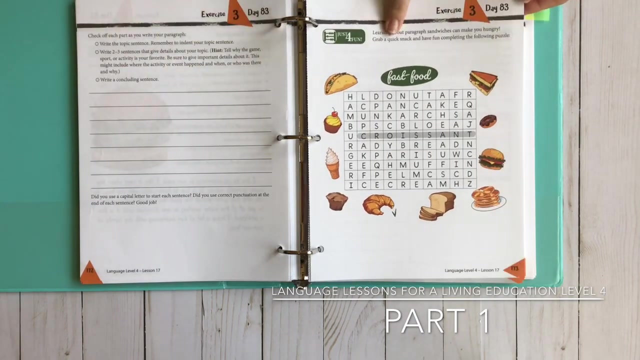 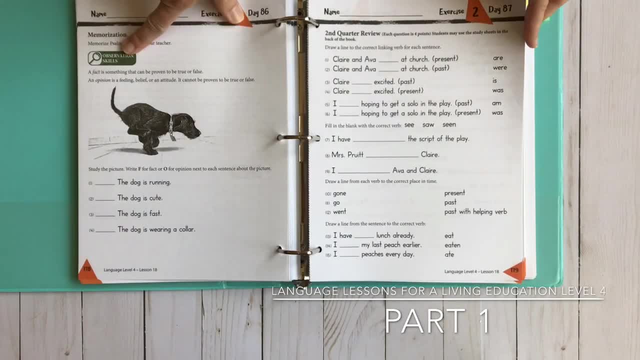 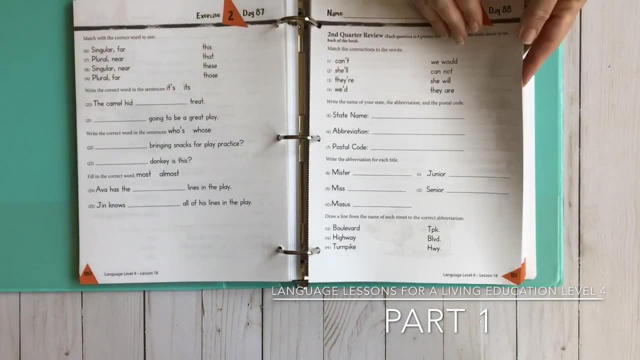 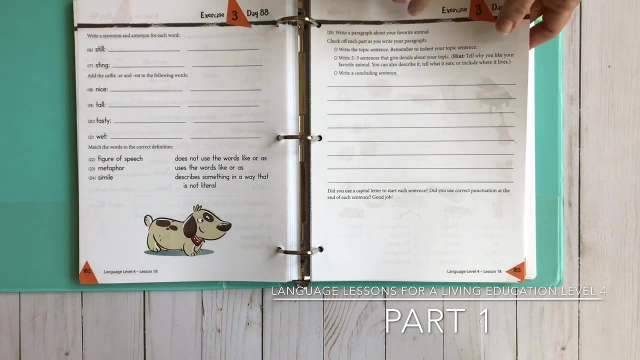 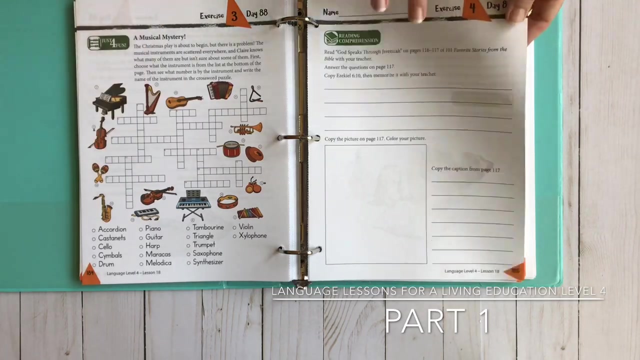 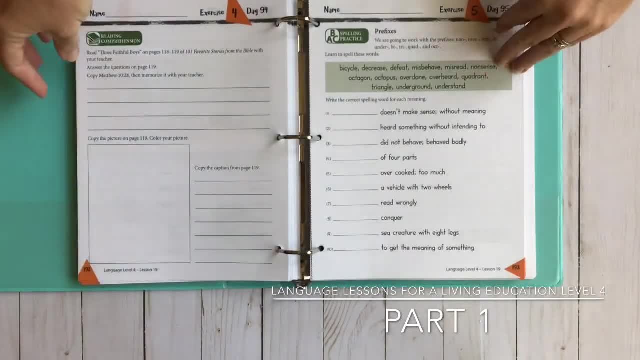 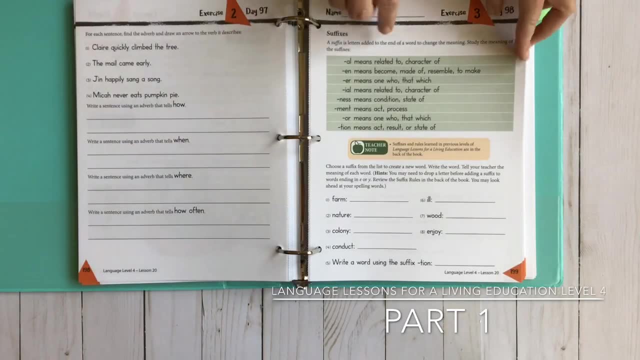 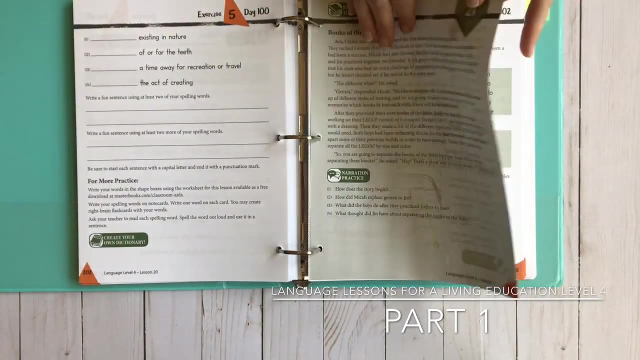 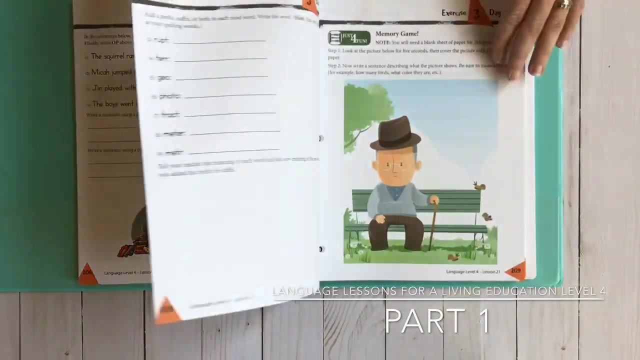 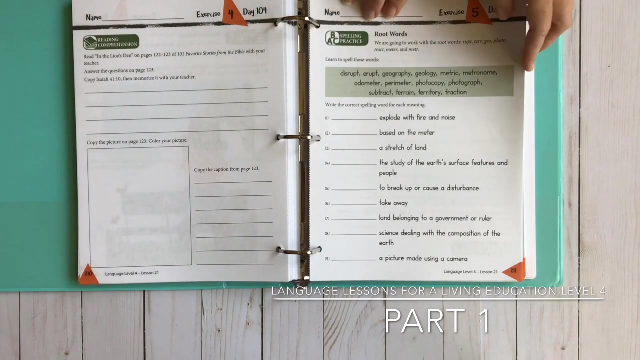 some prefixes. a picture study- you're in adverbs suffixes, your spelling practices with suffixes, some memorization- there's a memory game that looks like a lot of fun: to look at pictures and try to recall what's in them. Those are fun. Root words: nice, pretty. 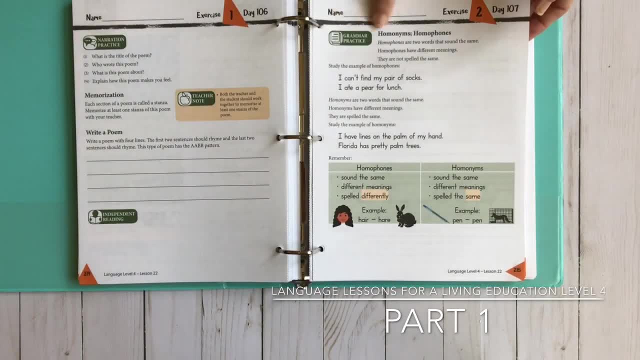 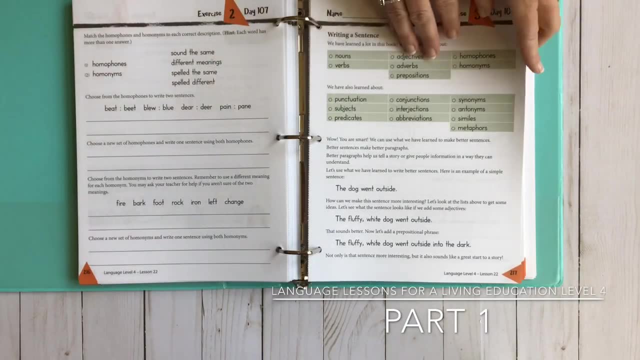 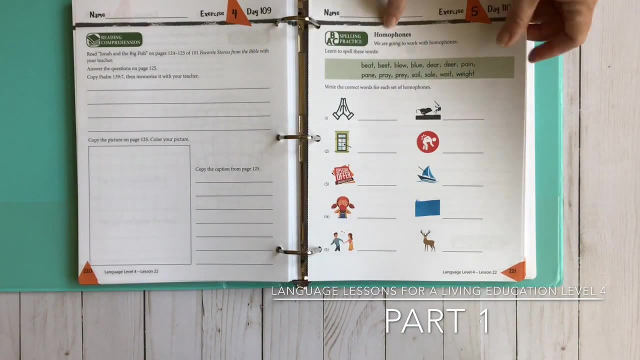 poem. Your grammar practice in exercise two for day 107 is homonyms and homophones. I like this just for fun, where they have to try to draw it. And then your spelling words for that week are homophones and they use little pictures. 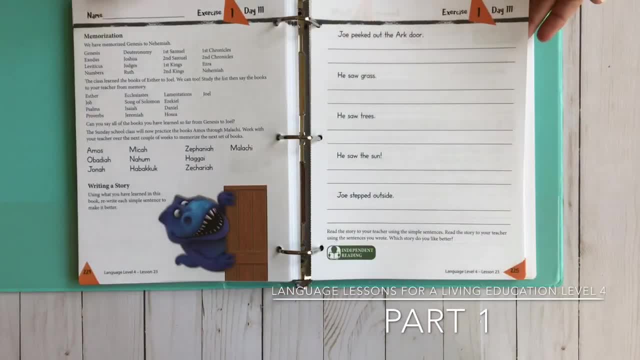 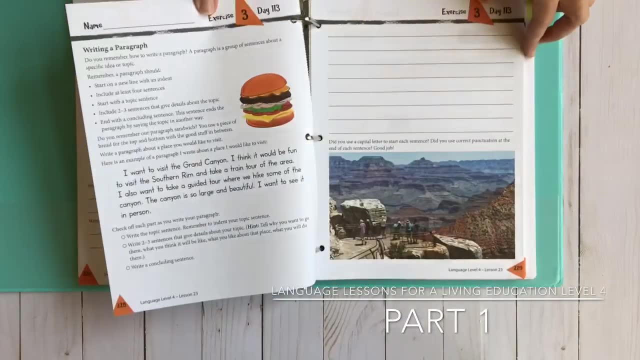 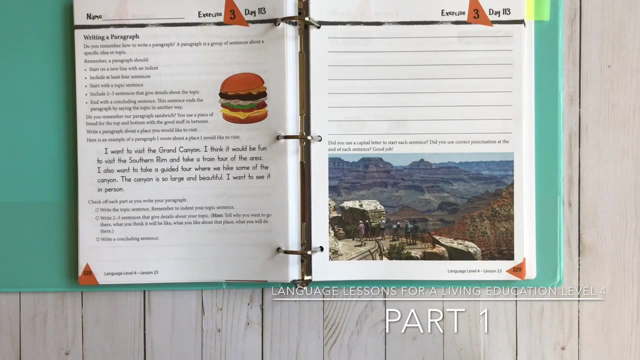 Reading Your books of the Bible memorization. Your grammar is still homophones. Your exercise three. here again you're looking. you're using that hamburger paragraph. using this picture, You're talking about a place that you'd like to go, like to visit. 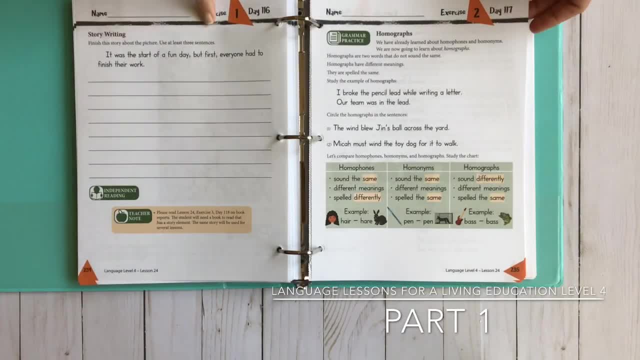 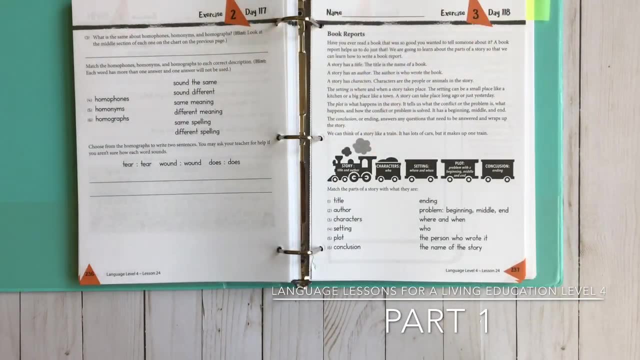 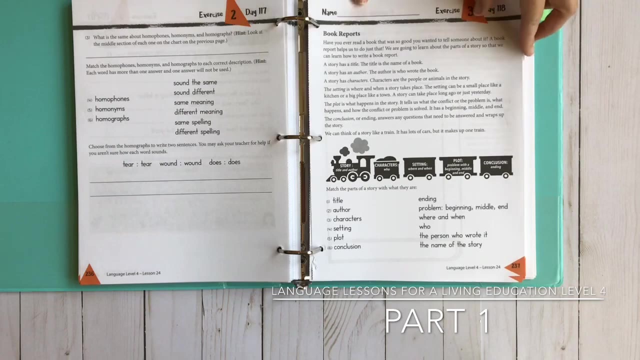 Here's another where you finish the story. Then they use how to write a story- Not just a writing prompt, but actually writing a story- so they give it to you like a train. You gotta have all these parts. So I do like that picture. 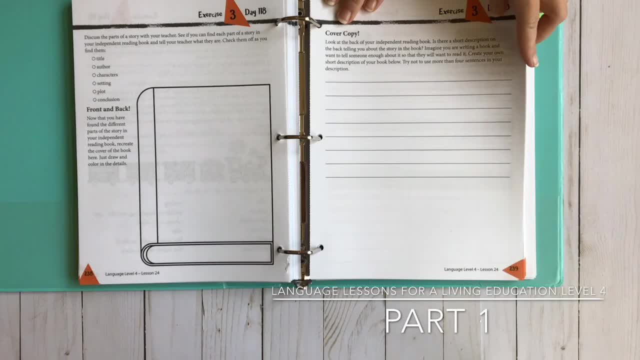 to help him. Another word search. We're all the way at lesson 25.. Kathleen Hayes, There is another word search, You dumbass. There's another word search: Three cave should. Here's another leg. you cut Name of the story. 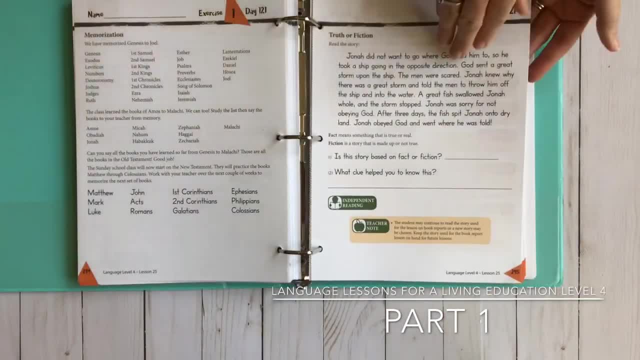 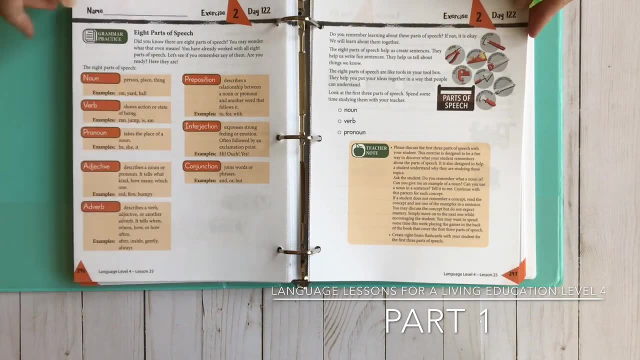 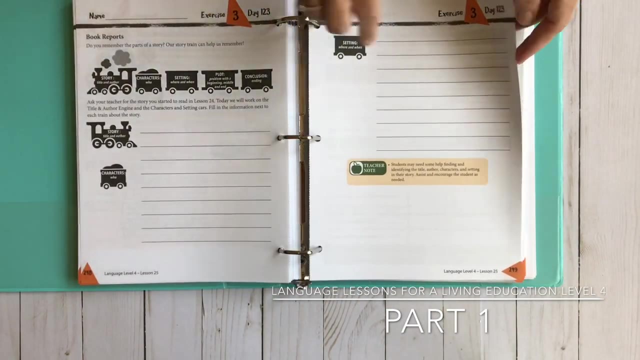 less than 25, so we're getting there. Just trying to let you see the whole thing because it's very helpful. Here's the eight parts of speech. This might be something you want to keep for reference. Keep it out so that your child can use it. and again you're back to the train, since. 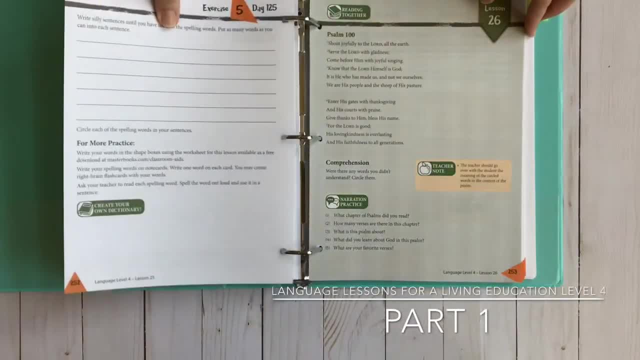 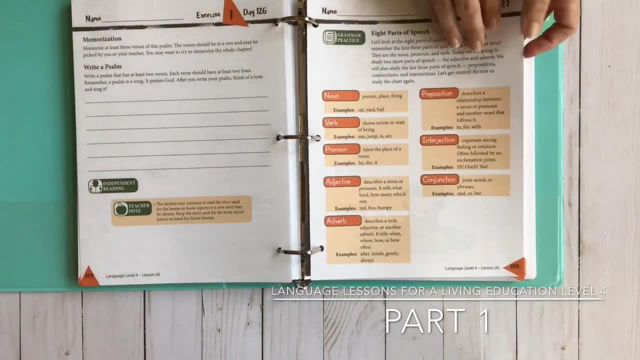 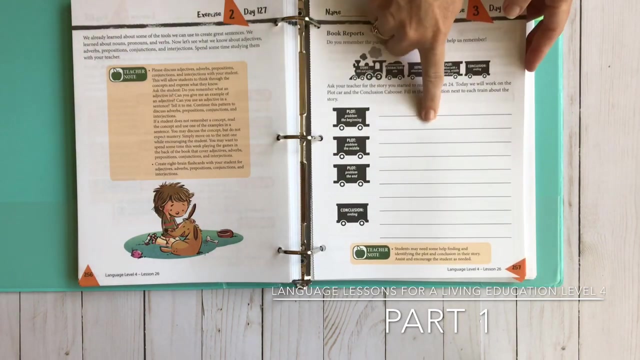 you're writing a story, You're going to write silly sentences with your spelling words. Here's the psalm. again Here's your review of the eight parts of speech. and then again you're back to writing a story and see again, they're not asking them to write a ton, They just want it to be. 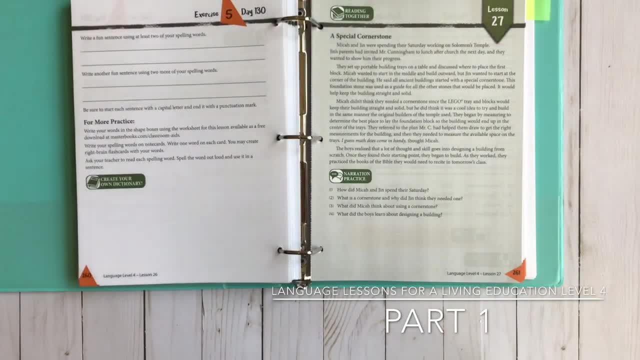 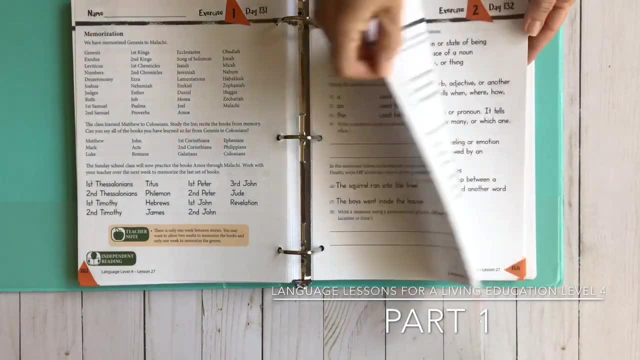 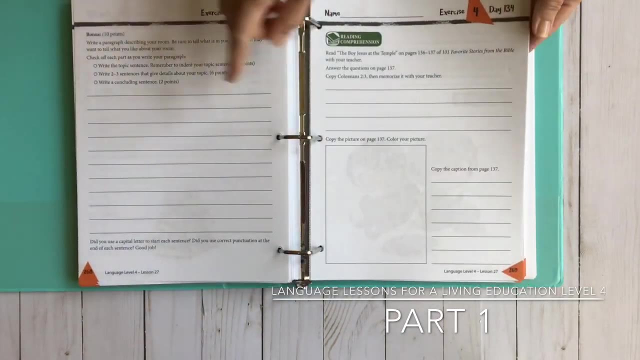 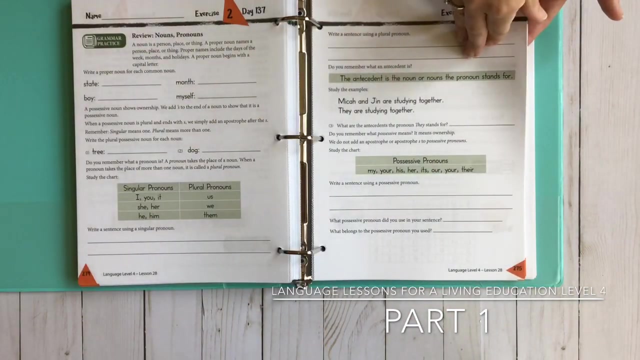 written well and that's important. You don't need. I don't think volume is important, as if it's written well. Here is another story, Some more writing. These are books of the Bible. again. Review of pronouns, review of sentences and punctuation. 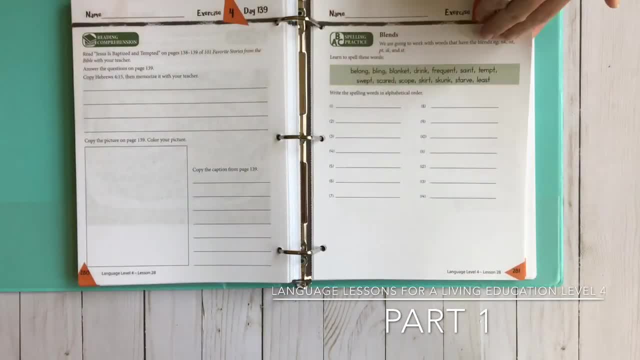 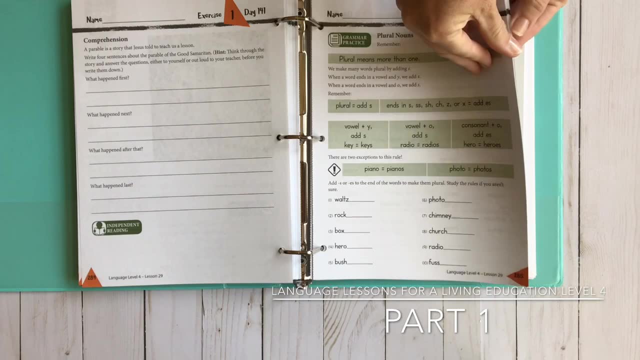 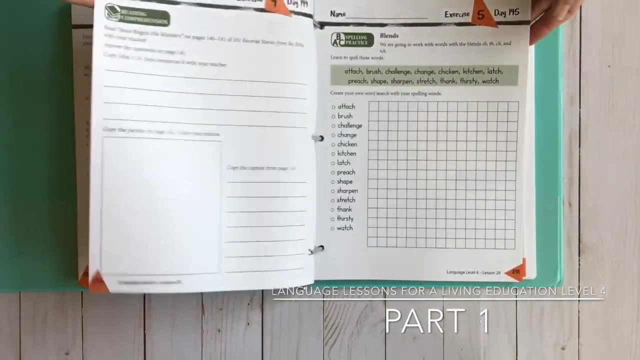 Another, just for fun. Another picture study. so we're up on lesson 29,. and we're still going strong. Here we go. Wacky word, fine time, That's neat. Now you're working on blends, Spelling words with blends. Here's lesson 30.. 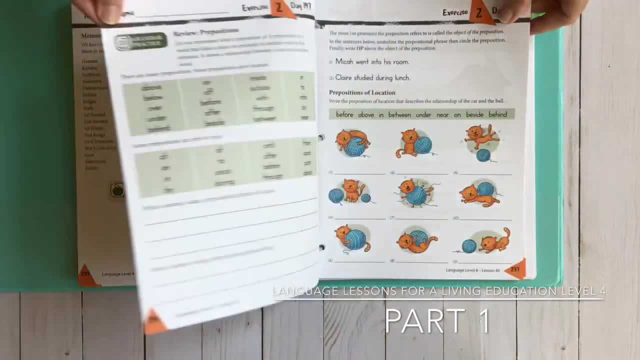 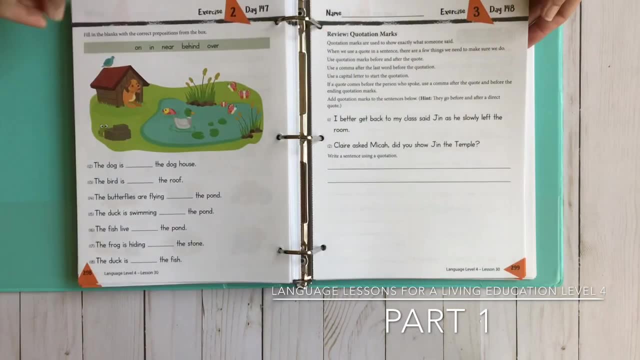 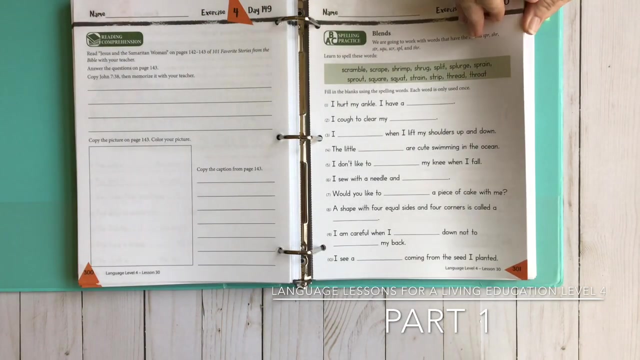 Here's review of prepositions. I like this little cat. That's really cute. Review of quotation marks, which is very helpful. My son needs practice with that and your words are blends again. Lesson 31,. you have a poem about the field mouse. 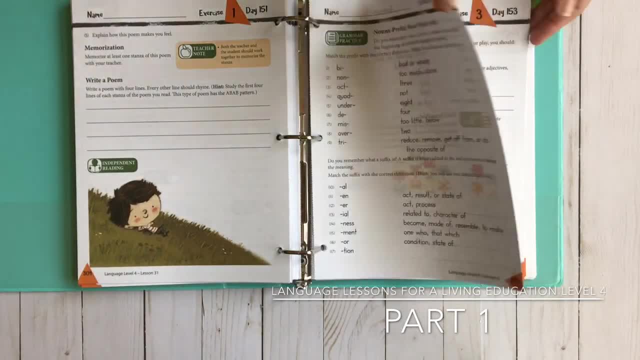 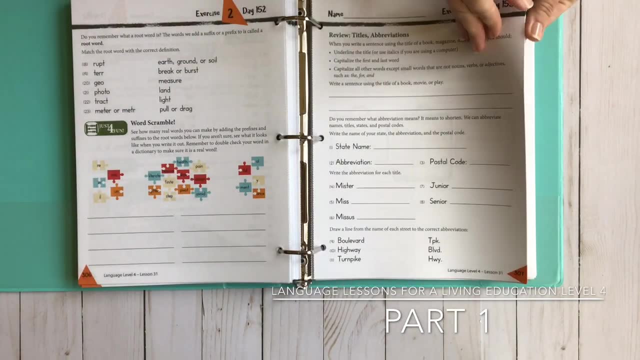 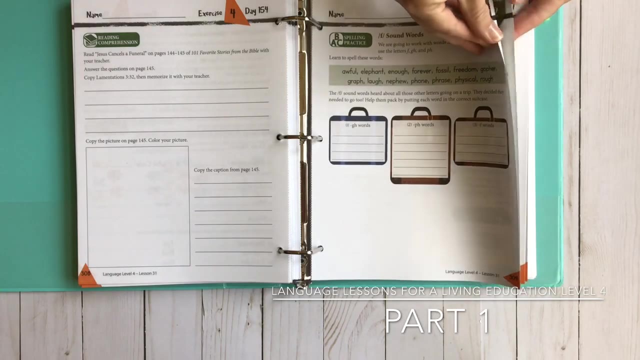 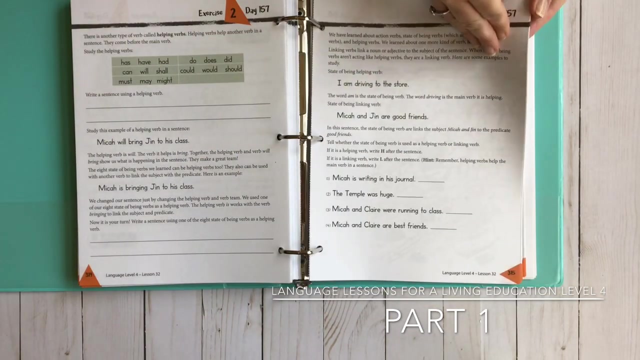 You're going to write a poem there. Grammar practice is nouns, prefix, root, word, suffix. You're going to review titles and abbreviations. Another story: Some mat work, Se 1942 to 1980.. Forties shorts. 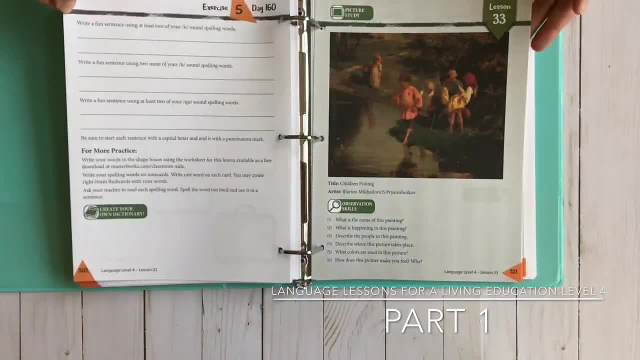 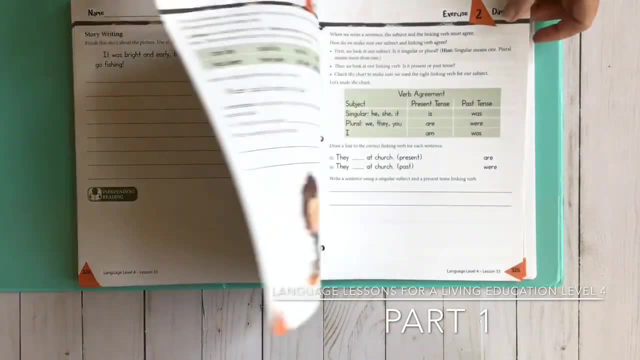 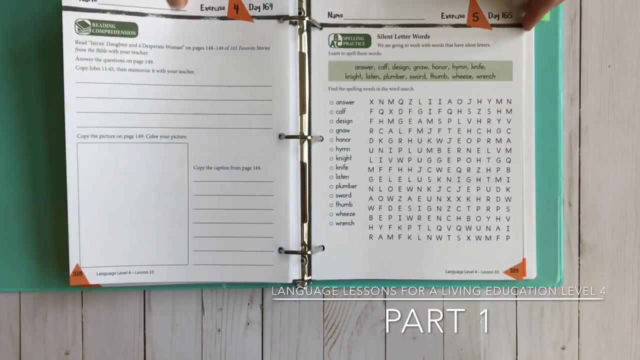 green, brown, orange. just very predictable. here's a picture page. you're gonna do a picture study. you're going to finish the story. you're gonna review verbs, going to review how to use the dictionary and you're gonna have a silent letter, words and you have. 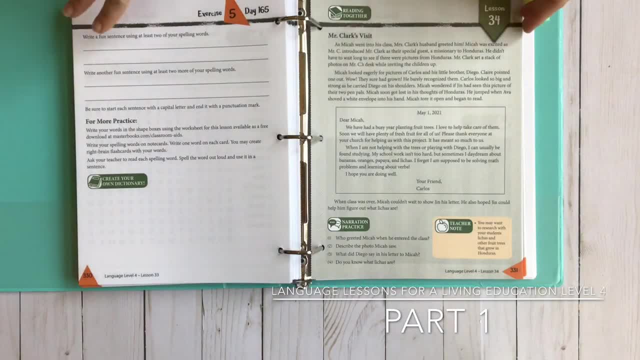 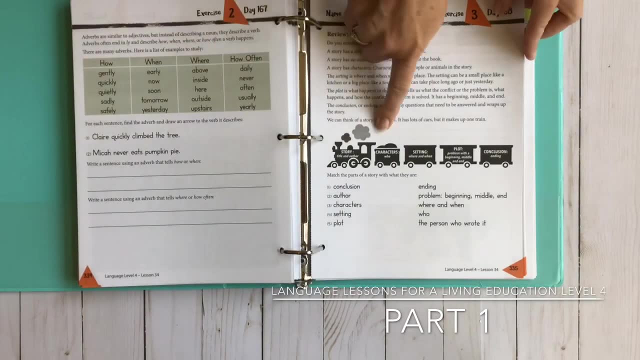 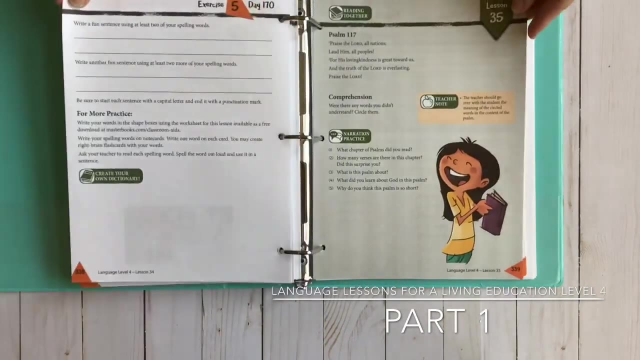 a little word search, so it's not always the suitcases sometimes that changes it up. here you're gonna read a letter. here's the train again so you can work on parts of a story. you have double consonant words. then you've got a song. some grammar practices: just review and 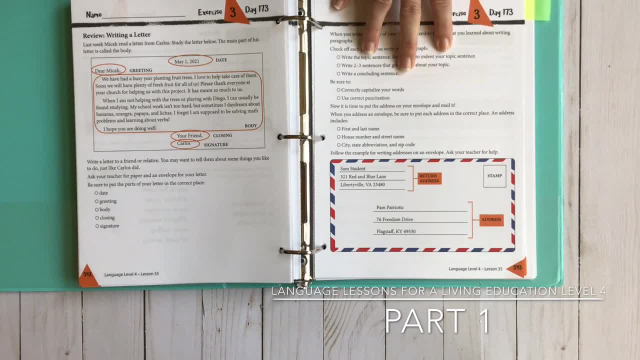 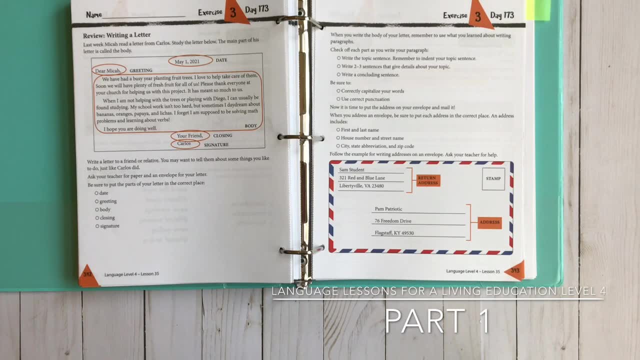 this. I worked at a co-op this year and we made a postcard and I had to give them instructions on how to address the postcard, so I thought this might be something that kids are missing out on. I don't know they're writing letters anymore, So I'm very glad that this is in here so that my son can learn how. 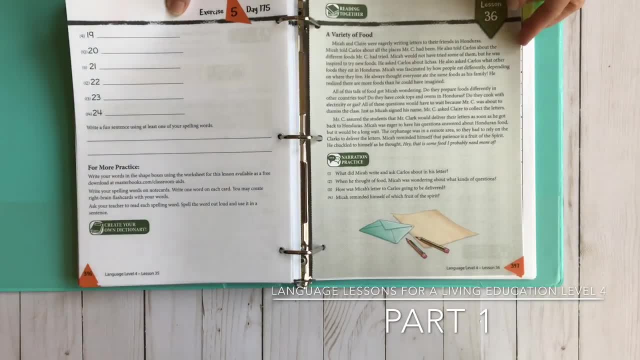 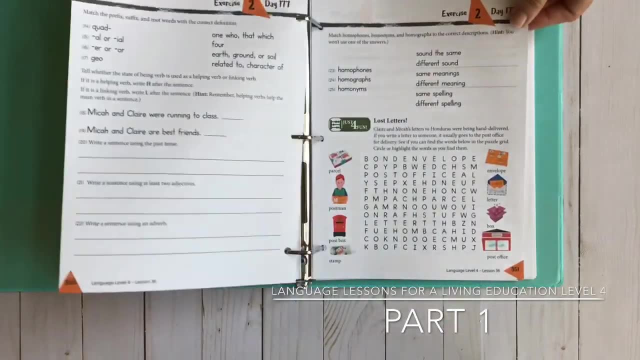 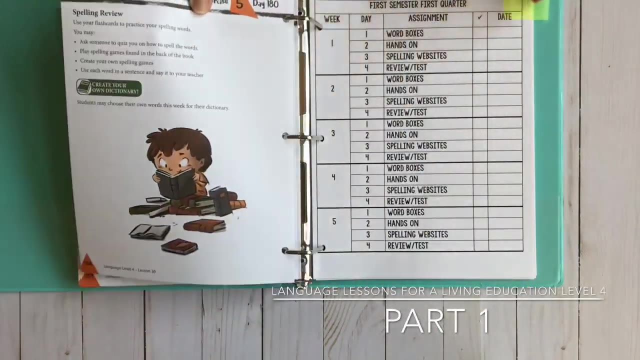 to do that All the way. at lesson 36,. you've got a story to read. an observation just for fun. Here's your fourth quarter review, And that's it. So what, this is my son's notebook. And then what? 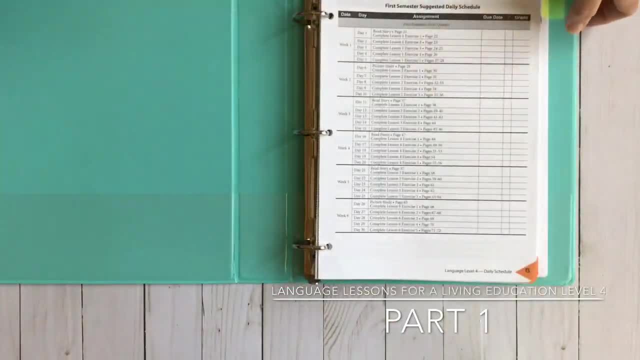 I want to show you is my notebook that I use, So that is his.